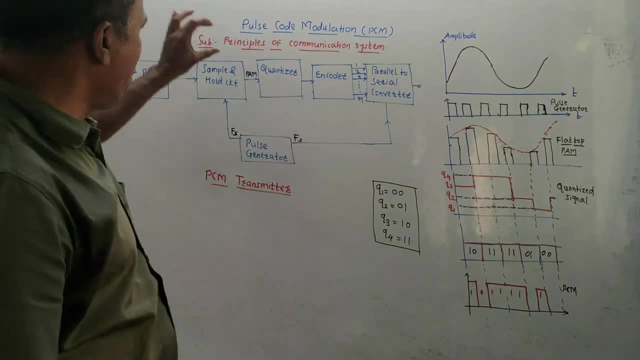 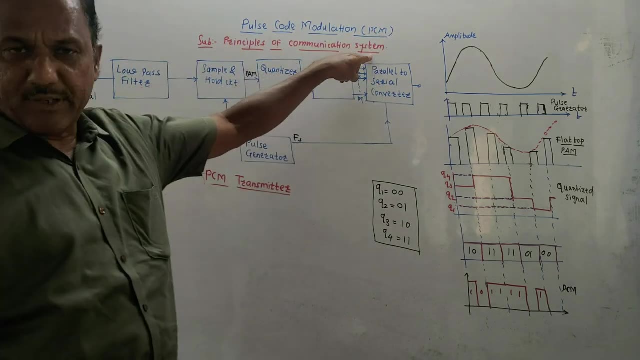 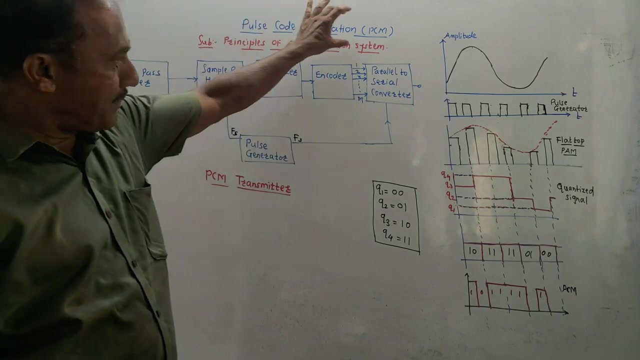 Hello and welcome back to this channel, Dear students. this topic is pulse code modulation, that is, PCM. It is the topic from the subject principles of communication system. In this session we will discuss the transmitter, receiver of PCM system, as well as we will discuss advantages. 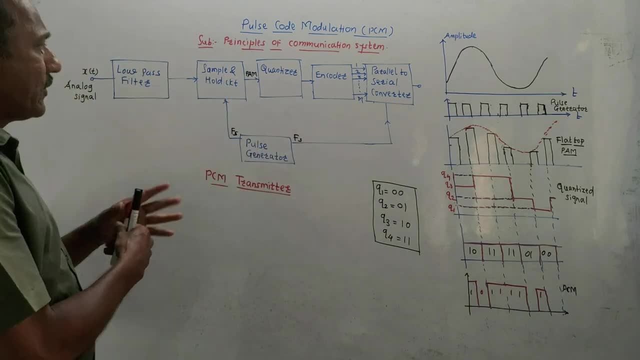 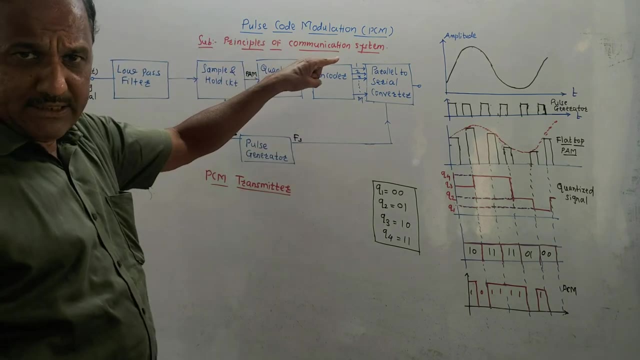 and disadvantages of this system. From the example point of view, you can expect a question like this: draw the block diagram of transmitter session or generator section of PCM system and explain its working, as well as for the receiver, same question: draw the block diagram. 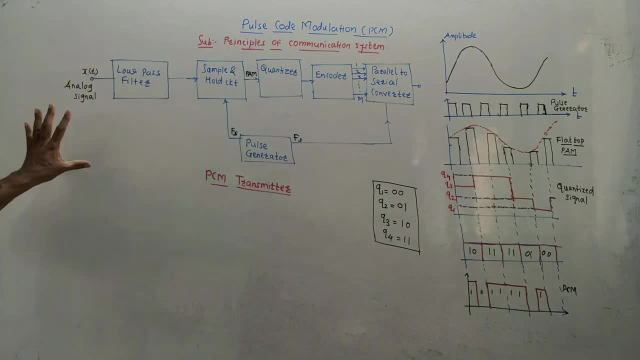 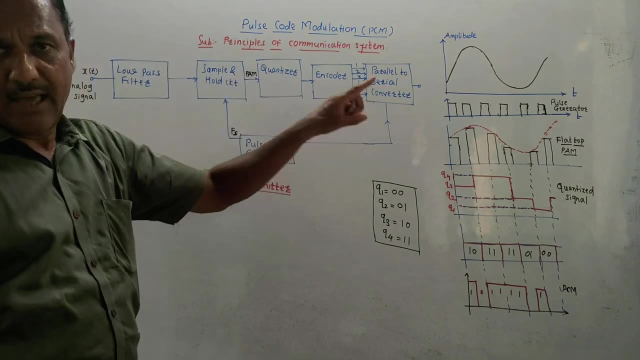 and explain its working. So, without wasting the time, let us start the topic. So this is the block diagram which is used to generate pulse code modulation signal, As the name indicates. at the output we are going to get different code words, So at the output: 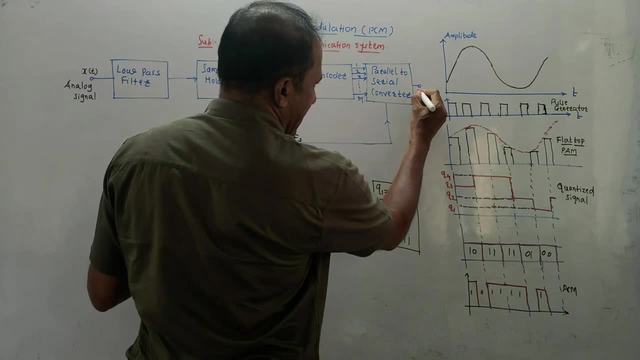 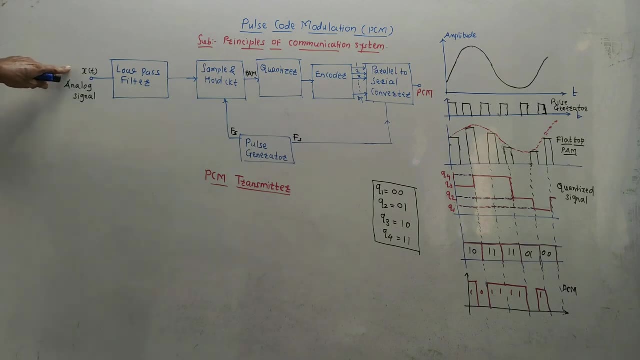 we will be getting PCM signal. This is the output of generator. Here I will write PCM, That is, you will be getting code words. Now see at the input. we are applying analog signal. Xoctane First block is low pass filter. This block is also called anti-aliasing filter. 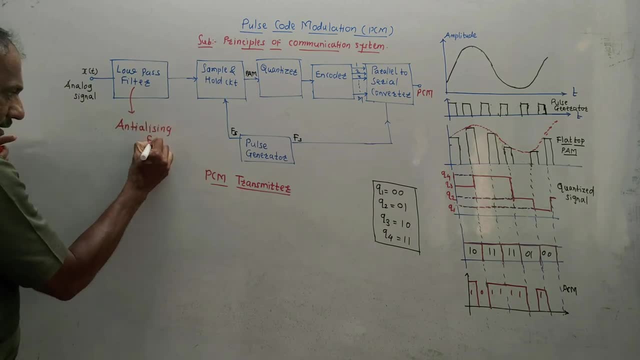 So this is again anti-aliasing filter. In the previous session we have discussed what sampling is. What is the function of anti-aliasing filter. So, in short, you will have to write the explanation of this block like this: This is a low pass filter whose cut-off frequency is denoted. 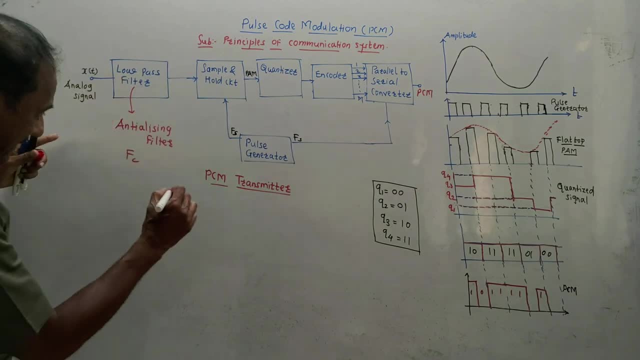 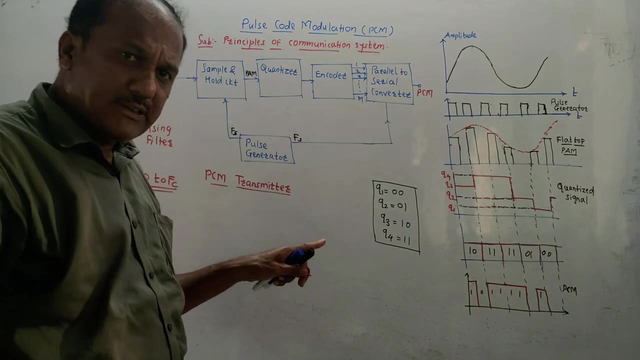 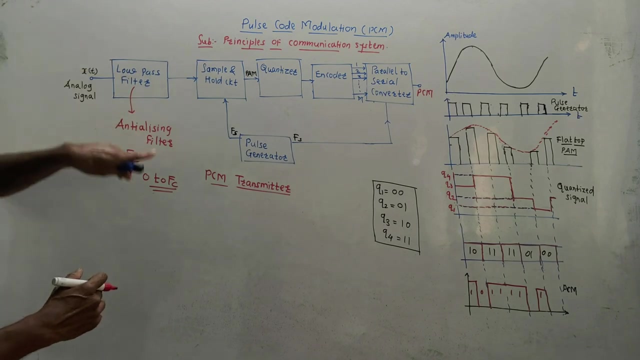 by fc. fc is cut-off frequency. This is a low pass filter. It will pass the signals from 0 to fc. The frequencies that are more than fc will be blocked, So 0 to fc signals will be passed. This is the function of low pass filter. Its cut-off is designed in such 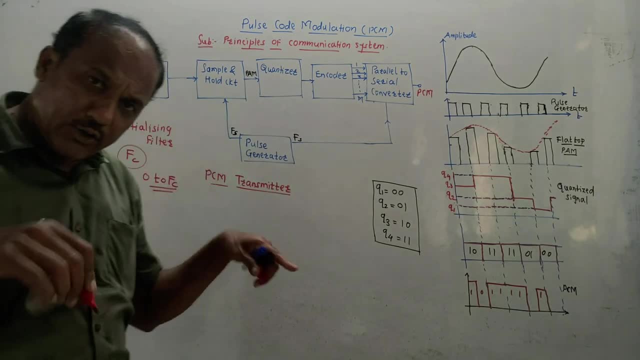 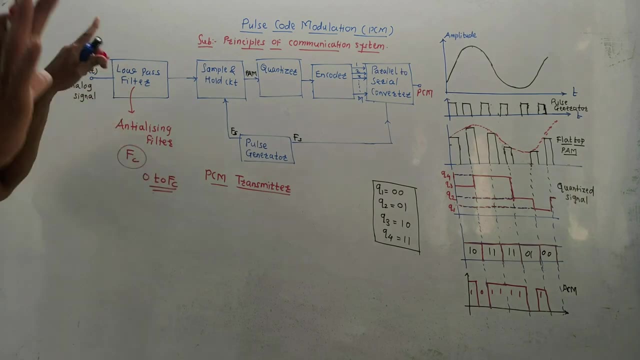 a way that it will avoid the aliasing effect, So it is also called anti-aliasing filter. We know that aliasing is mixing of signals, So it is avoided by using this low pass filter or anti-aliasing filter. Now the second block is sample and hold circuit. 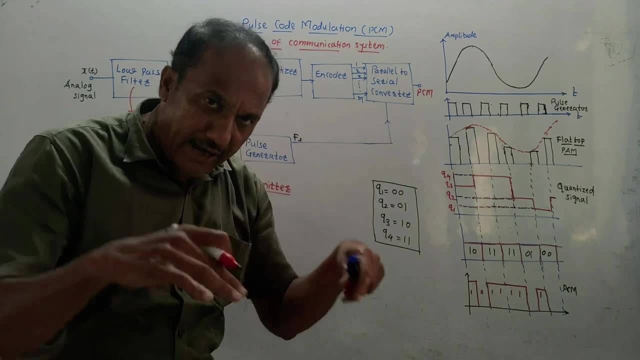 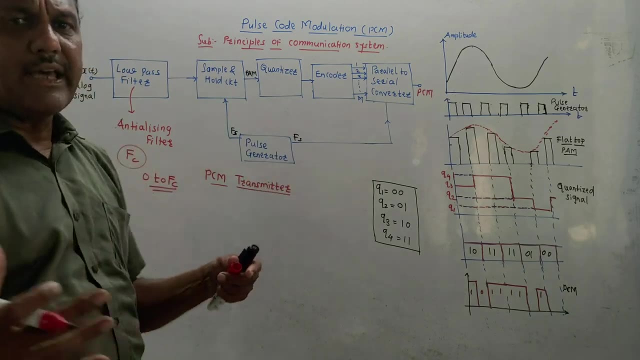 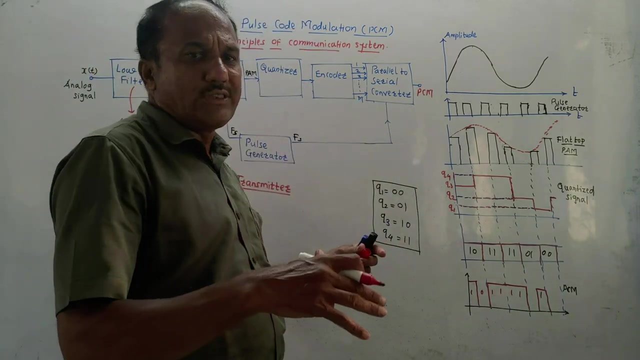 The major function of sample and hold circuit is convert analog signal into discrete pulses, Discrete signals, Discrete signals, Discrete signals. Now look, We have learned in the video about sampling: what are the types of sampling, what is the sampling and all that. If you have not watched that video, please do watch. 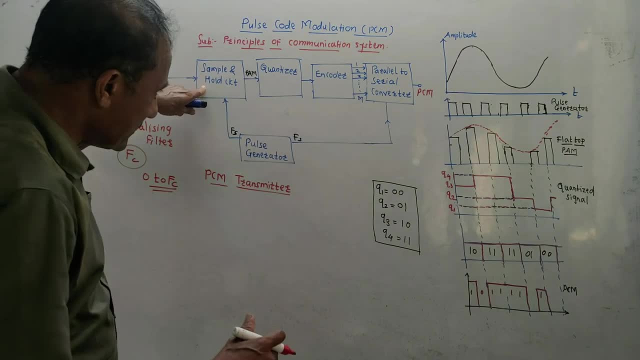 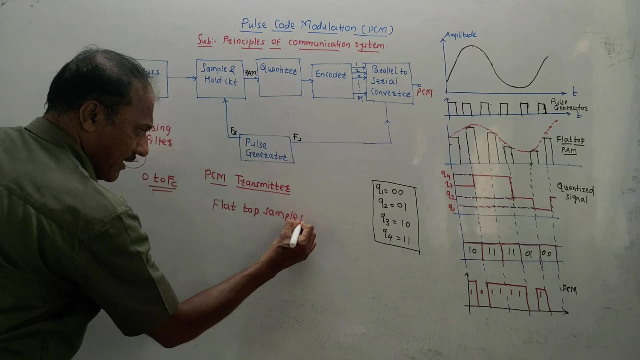 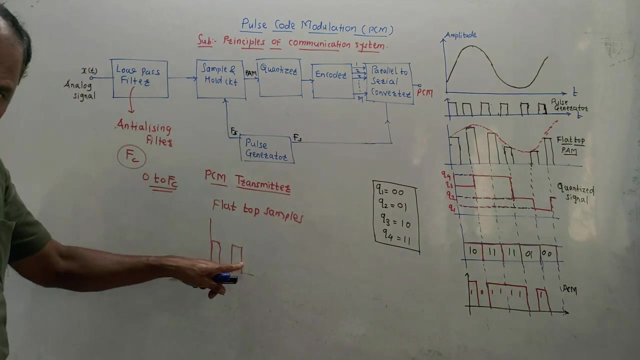 that video. The sample and hold circuit that we are using here produces the flat-top sampling. It is flat top sampling. Flat-top sampling means that in output we will get pulses like this: After sampling, analogue signal will be converted into discrete, converted into flat top samples like this. so this is the function of sample. 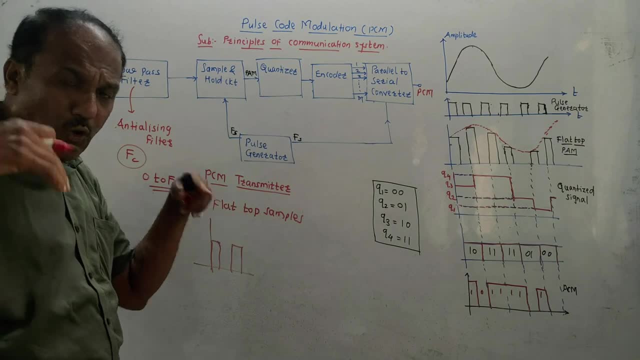 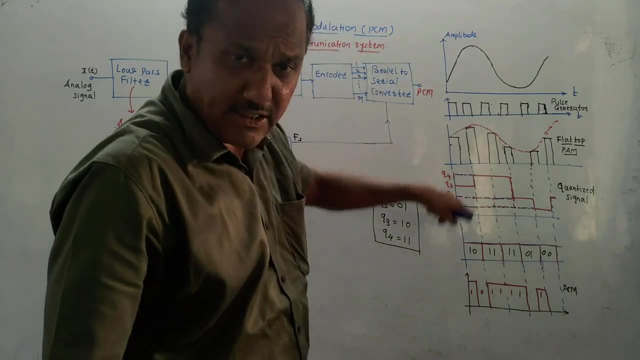 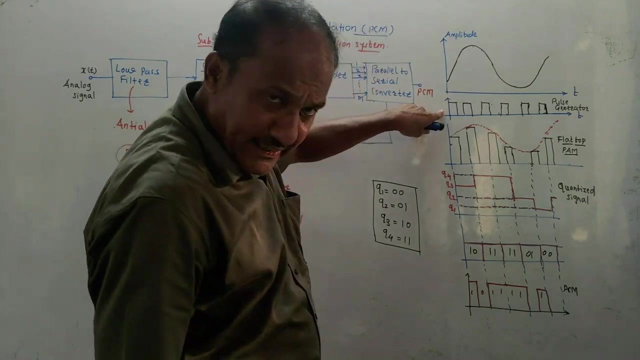 and hold circuit. it's like a reference a year. but you need to apply train of impulses. so for that pulse generator is used up, there is diagram a: many decay. these are the corresponding waveforms, yet input analog signal and this is assumed signal of age of second diagram. that is the waveform of pulse generator. 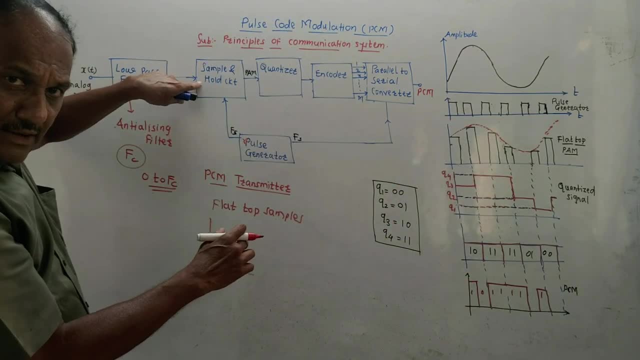 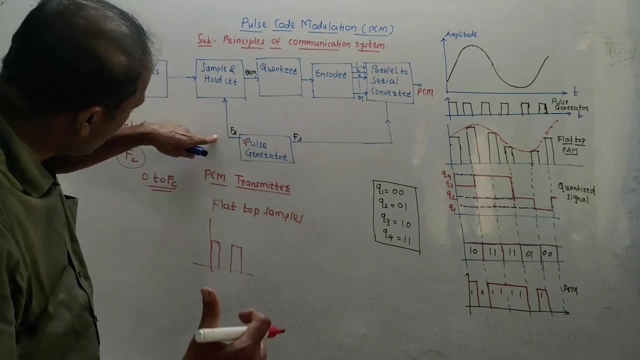 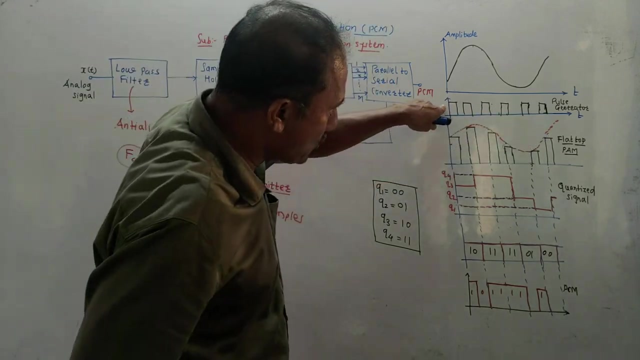 that's a very bad sample and hold circuit. function a to convert analog signal into discrete signal is killing. which pulses change for the operation of the sample and hold circuit. these pulses means the output of pulse generator. so it's got your put. I have shown it over here. its frequency is s? s we have. 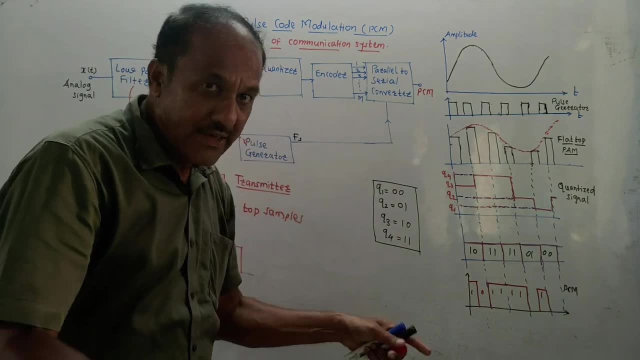 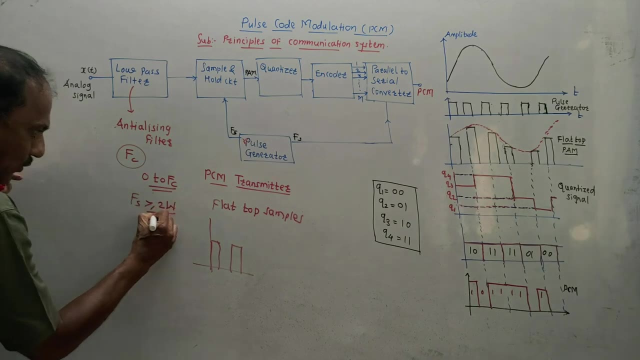 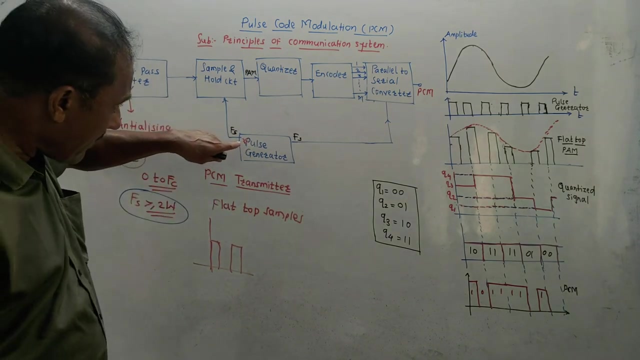 already learned. fs is called sampling frequency. yeah, we have local mention, Carnaval. a key fs should be greater than or equals to 2w, where w is maximum frequency contained in the signal. use your requirement a. this requirement is necessary in order to avoid the analyzing error or analyzing effect. so, accordingly, pulse generator generates the pulses. 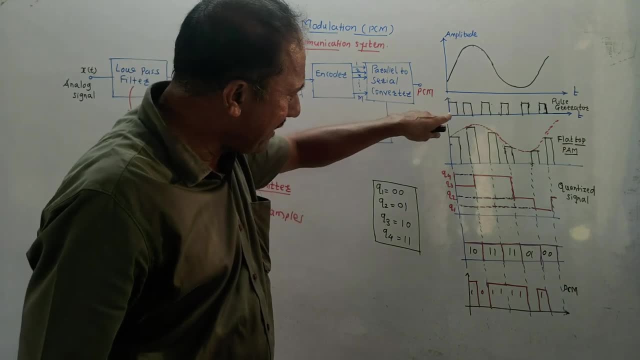 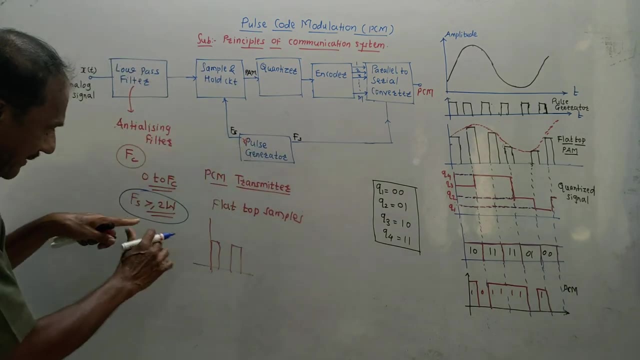 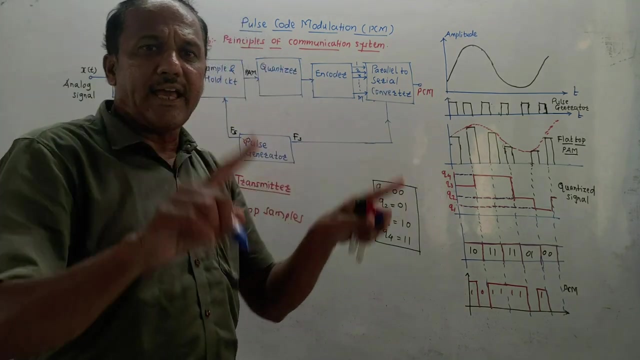 yejo, many is diagram a decay. hey, these pulses are having equal amplitude and equally spaced. so its frequency is ssfs is called sampling frequencies. I told you this condition is compulsory. fs should be greater than or equals to 2w. it is also called Nyquist criteria of the sampling. if fs is. 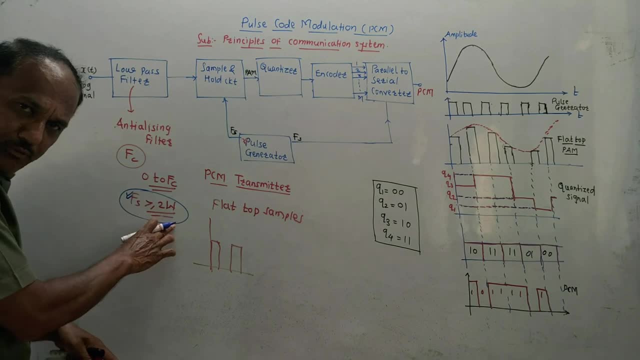 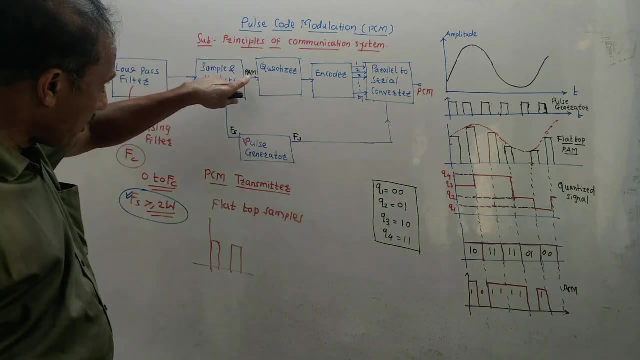 equals to 2w. exactly, equals to 2w. it is Nyquist rate of sampling and according to sampling theorem, value must be greater than or equals to 2w. okay, next block output of this sample and hold circuit is PAM signal. we have already. 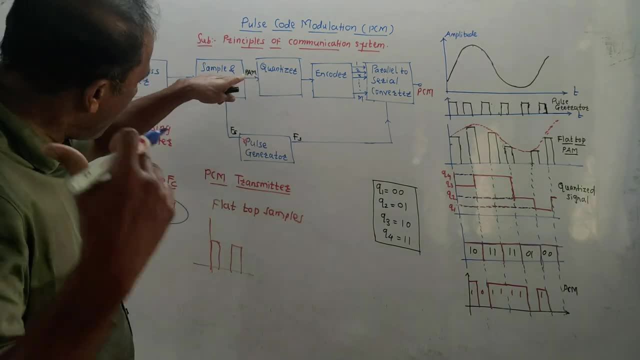 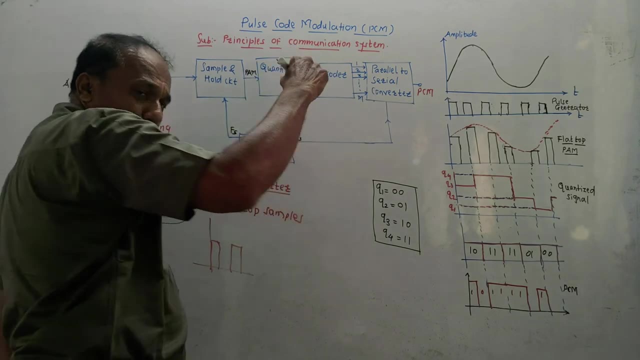 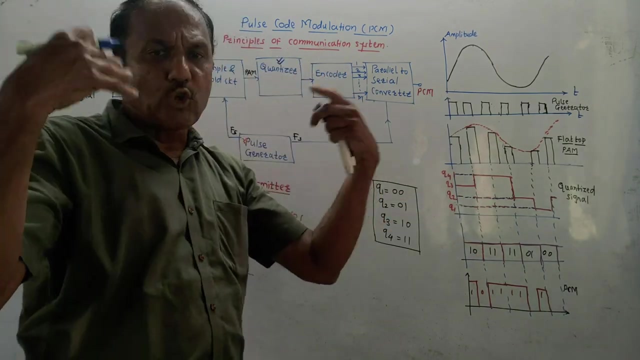 learned in last unit, PAM is pulse amplitude modulation. so at the output of sample and hold circuit you are getting PAM signal. yejo block hai quantiser ye hum log naise unit mein detail mein learn karne waale hai presently is request ka answer. likhte waktu what you are supposed to write. quantization is a process. 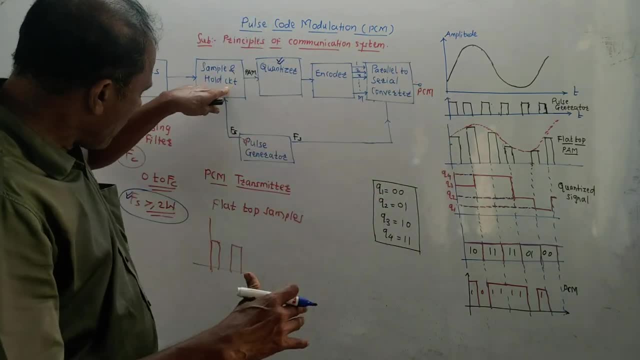 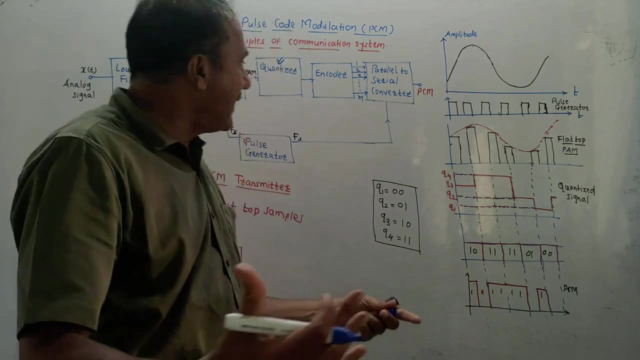 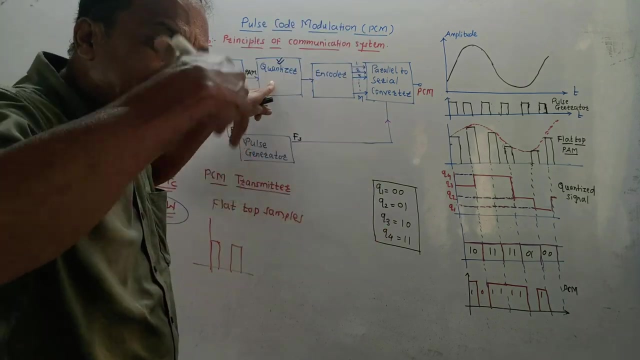 of approximation. matlab jase output of the sample and hold circuit contains many samples to osap samples. process karne ke lie bandwidth jyaada legke kar ye kam karne ke lie quantizer use. I am saying this very briefly about quantizer because it is the detailed topic which we 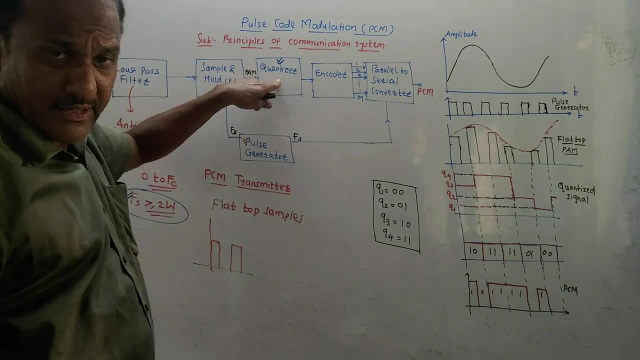 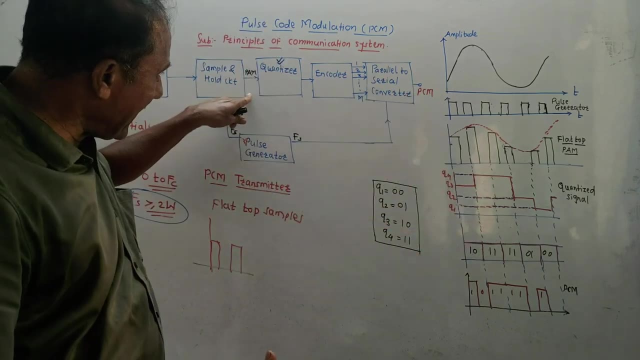 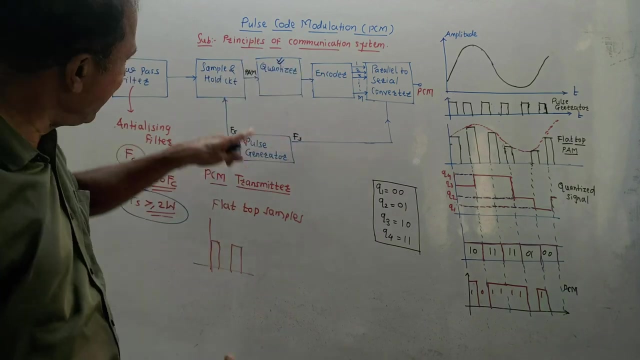 are going to cover in the next session. alright, so in its explanation you just have to write: quantizer is the process of approximation, so all the samples are coming. we will select a particular quantization level means we will consider a particular level. we will not be selecting all the samples which are getting at the output of sample and hold circuit. so 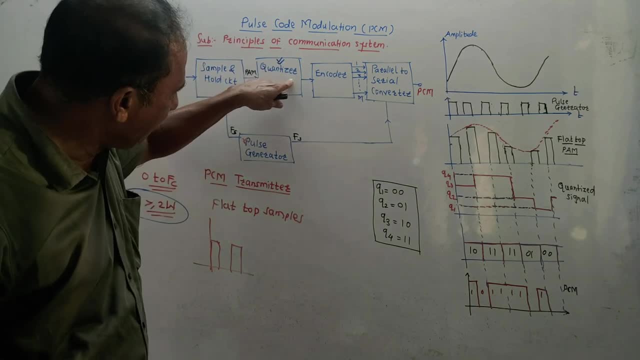 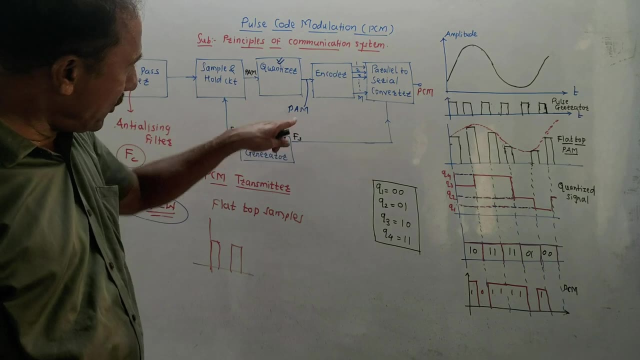 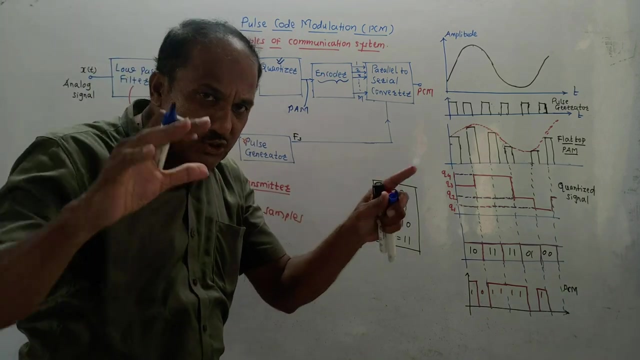 approximation is the function done by the quantizer. so at the output of quantizer you will get quantized to palm signal, that is, pulse, amplitude modulation signal, which is quantized in nature. next job block, that is encoder. as the name indicates, it provides code word, so different code words are generated. we know that the code words are in the form. 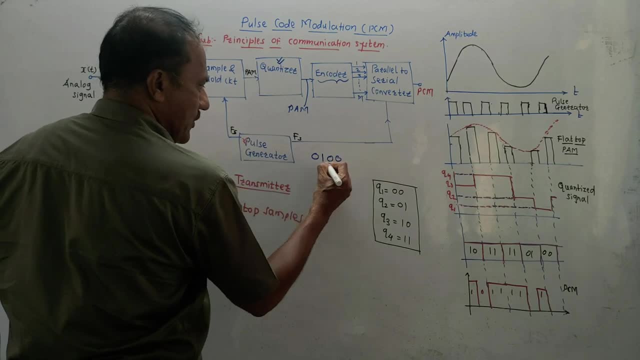 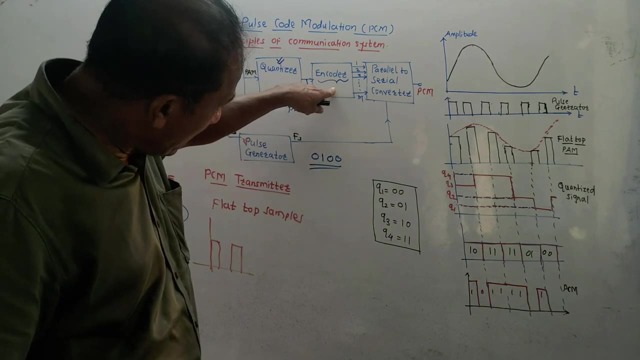 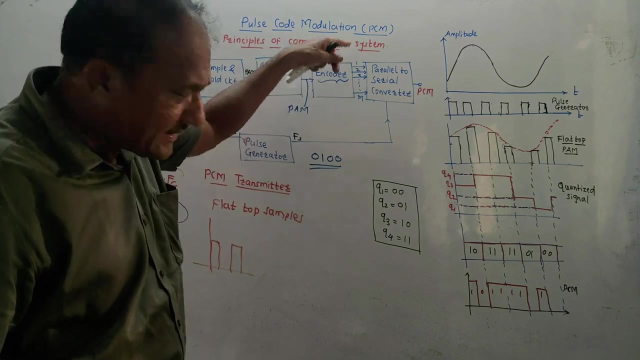 of binary bits, for example 0, 1, 0, 0. it is one of the code words. so function of encoder is to generate the code word. but the output of encoder is in parallel form: one, two, three upto m, so getting m number of bits at output. but for everything you might. 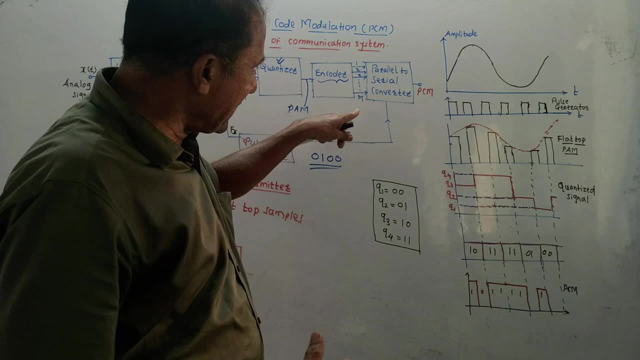 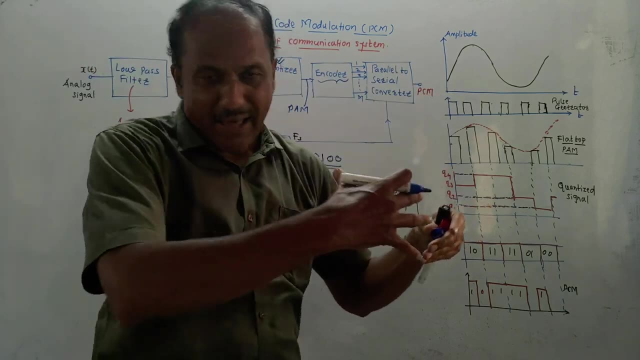 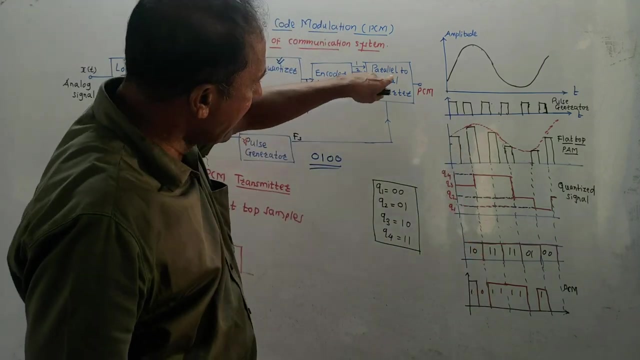 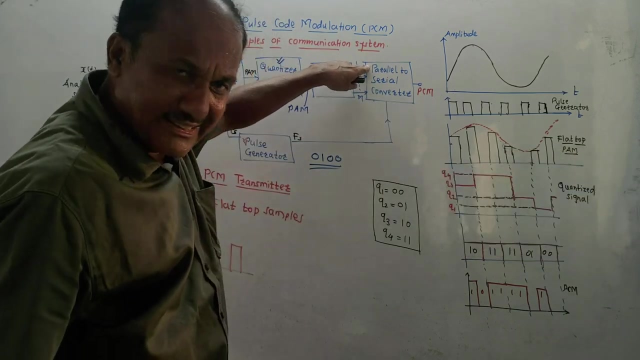 need a separate channel to transmit this data or it increases. if you want to send the like, this encoder output is a parallel form, parallel data you want to transmit through any channel width will be increased is the next block is parallel to serial converter but before transmitting it through some channel, the parallel things are: 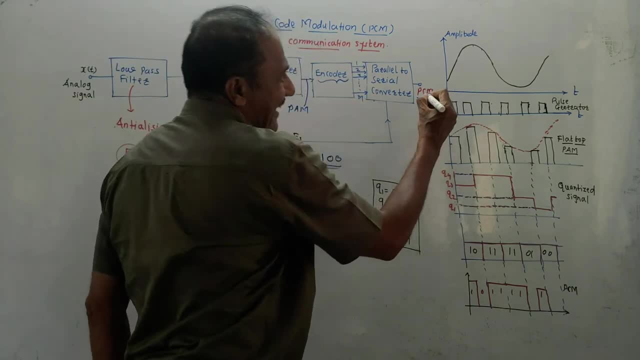 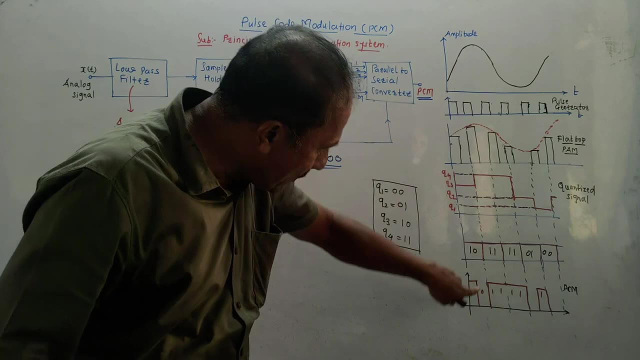 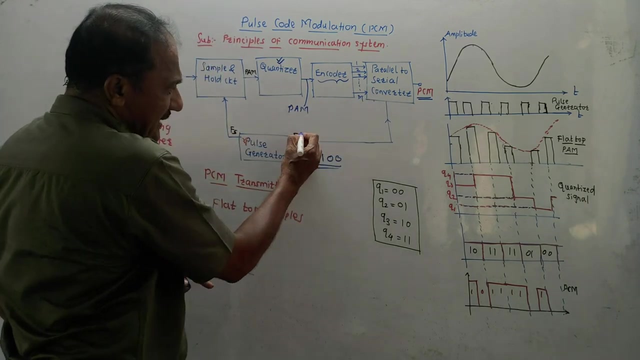 converted into the serial form or you have a output mill right. that is pulse code modulation to commit code word. may signal go convert here. but the analog signal that was for a stack, a codeword may convert here. may explain: current up long go up is clearly a reference signal, like I got, so same reference. 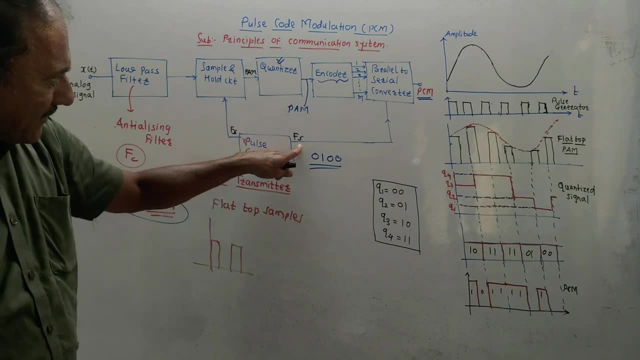 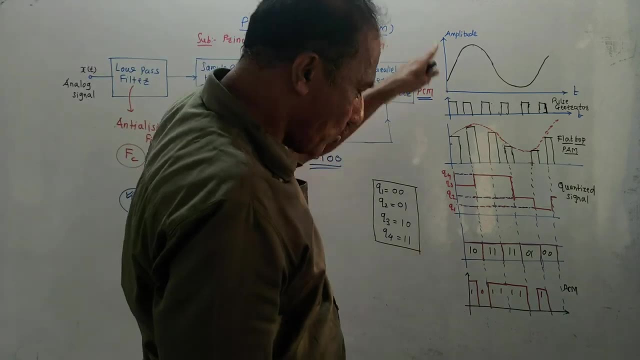 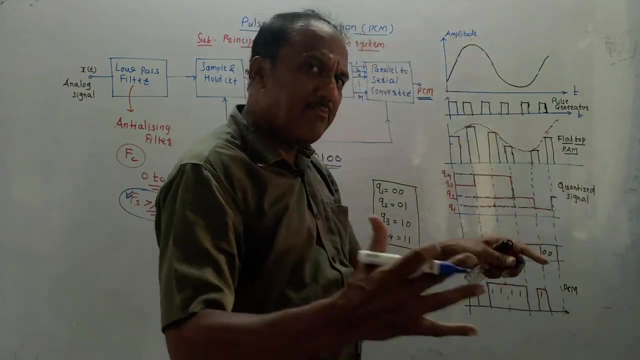 signal is the signal of pulse generator having frequency. fs is applied to this parallel, parallel to serial converter. okay up, what is this remaining? what are these remaining waveforms? the same, yeah, continuous signal X of T, just come with a codeword may convert, can I? PCM means pulse code modulation as a signal. 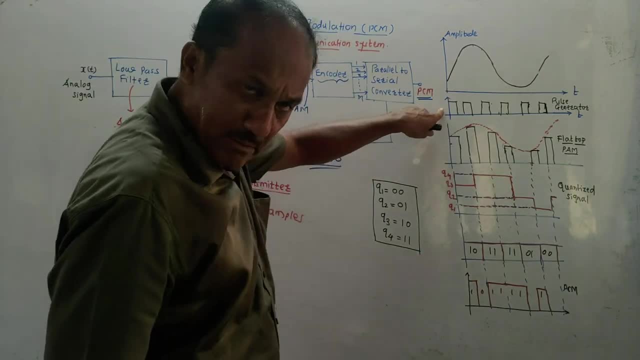 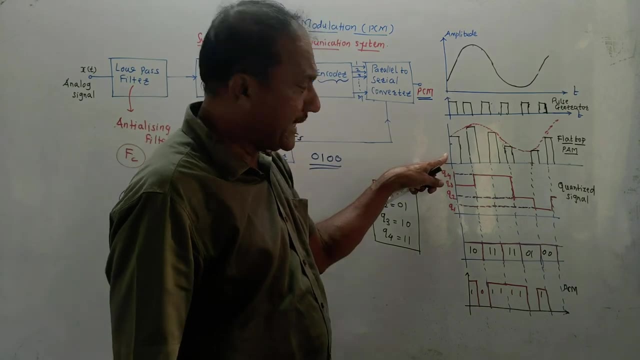 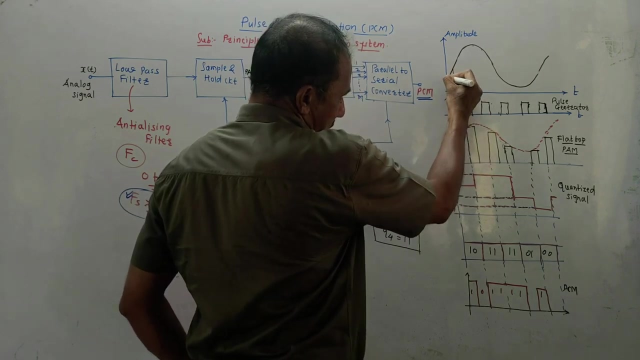 become a tonight. this is the output of pulse generator. yeah, I'm going to already discuss here whose frequency is fs next, yeah, Joe put it. this is output of sample and hold circuit. so they say they go. yeah, be a juice signal, a, a pulse, a so particular portion corresponding to this. 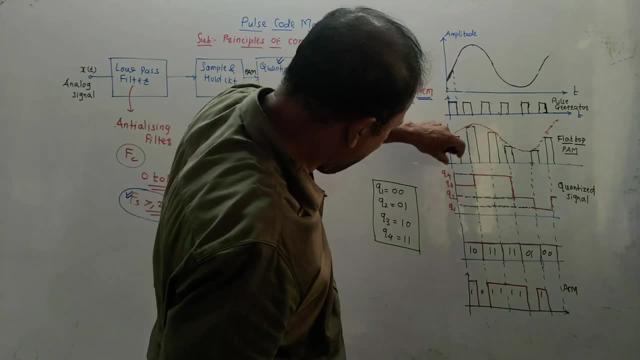 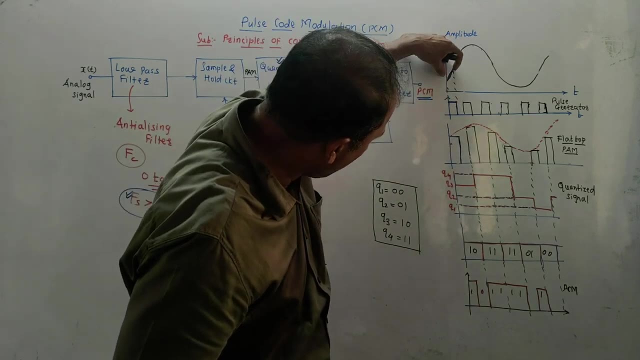 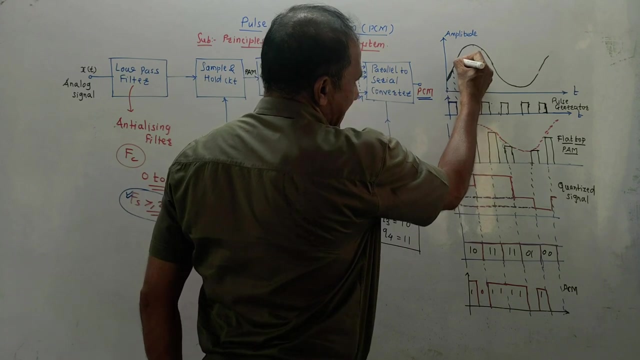 pulse. this is the particular portion your portion select can again add the output. you are getting the output pulse like this: this is called a flat top sampling mother job. a pulse a with no portion input signal: casita, yeah, but you will get. you will be getting the pulses like this second. they say: yeah, pulse a. 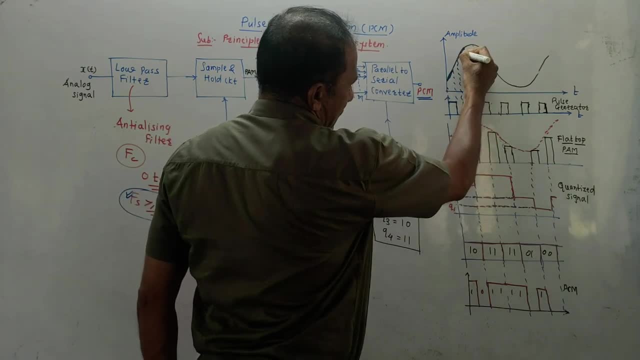 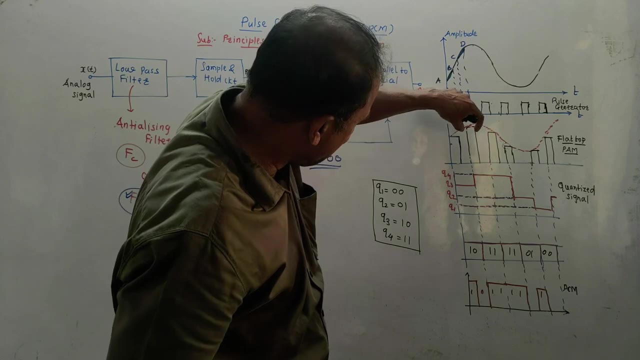 is a related amplitude. the coin put signal car. yeah, yeah, portion, suppose this. this portion is from a to B, this portion is from C to D. so C to DC related jitna, with the jitna a amplitude ahead with my amplitude in flat, me leg up no. 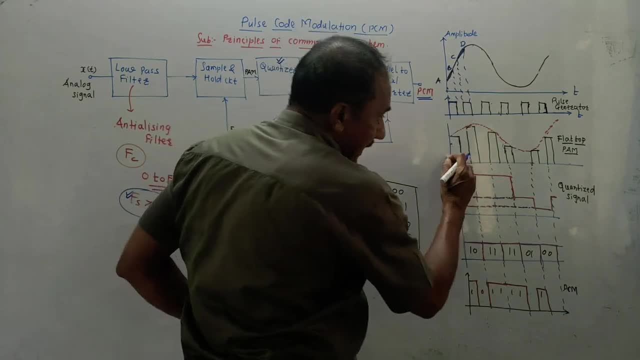 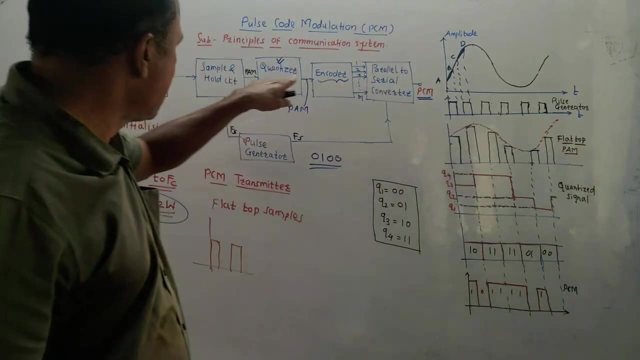 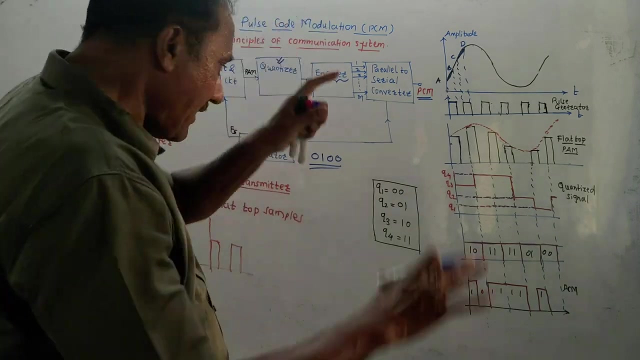 more with three men say so, yeah, well, a pulse mill, mill, Jada, likewise you will be getting different pulses, you, Joe head, that is. that is the flat top PAM, which is the signal you are getting at the output of sample and hold circuit. now main block, a quantizer is example. in is diagram made for this particular signal. 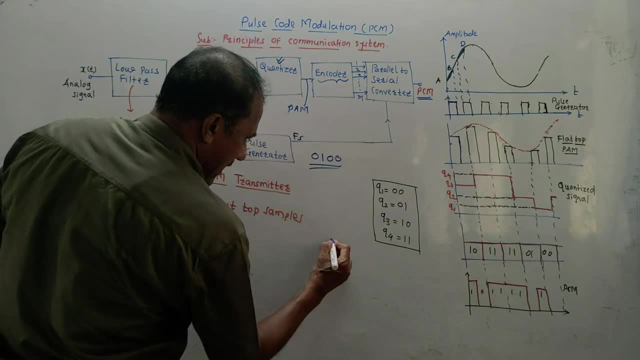 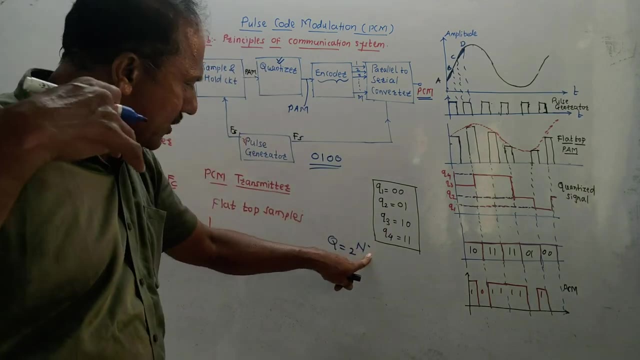 I have assumed few levels. actually, relation is: Q is equals to 2, raise to n Q. but the quantization levels and what the kidney bits use, curry, suppose I'm. look though we choose curry, a level, indicate, currently does a minute. but a quantizer, matlock, pura, pulses, select, make a net. 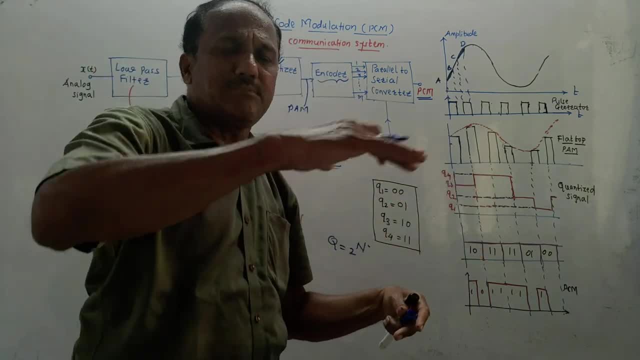 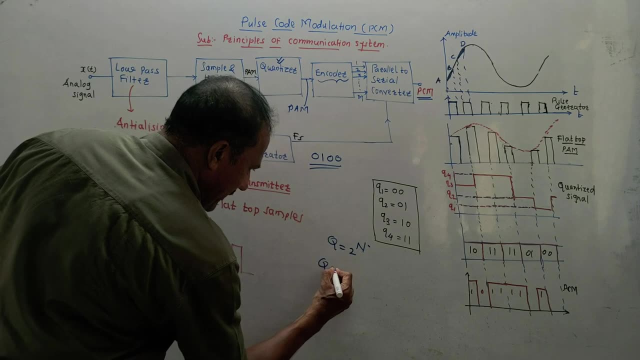 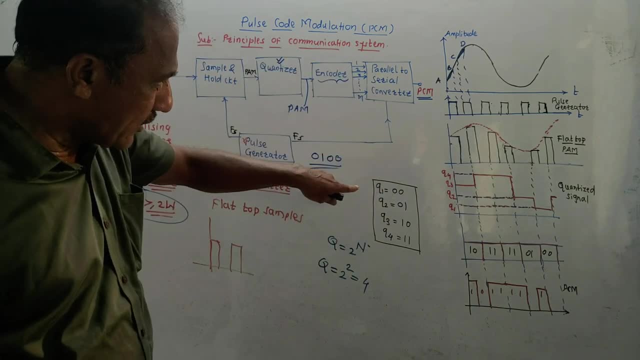 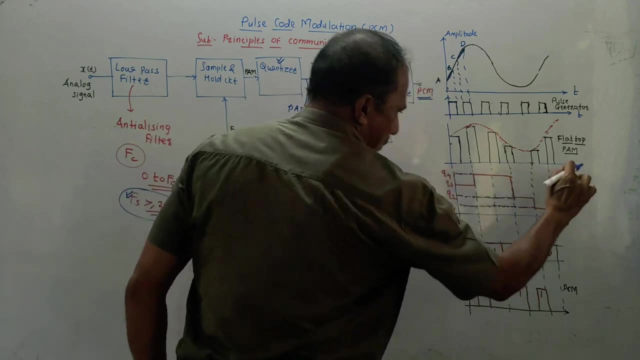 to raise to 2, that is four. so when I assume here the levels, quantization levels are Q 1, Q 2, Q 3, Q 4, so accordingly I have marked these levels Q 1, Q 2, Q 3 and Q or a bigger diagram drop as a connoisseur. 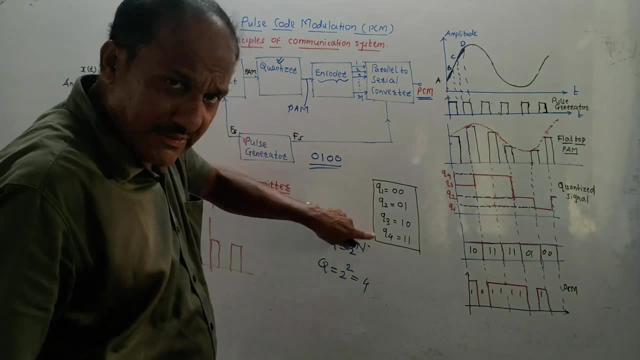 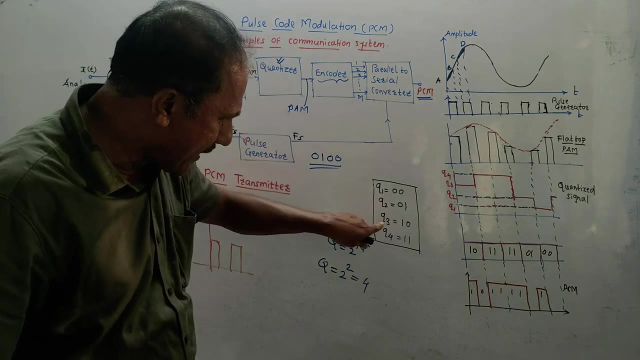 quantization cup. this is charge quantization level a year. clear cut assumption. hey, so I'll be assigning some bits like Q 1 to 0, 0 to 2, 0, 1. Q 3 to 1, 0, q4, kill a 1, 1. yeah, bits of low only assign key quantization level. go up. 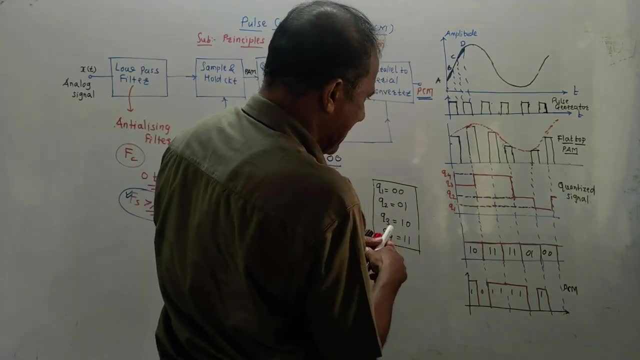 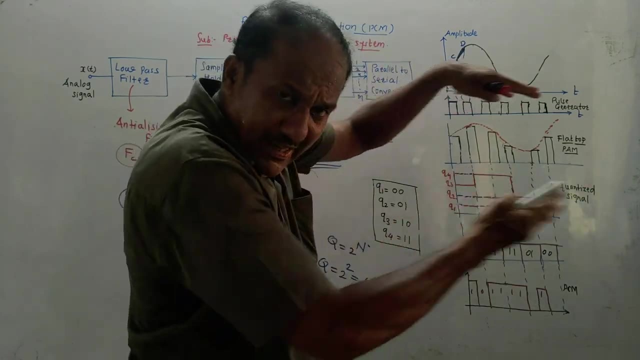 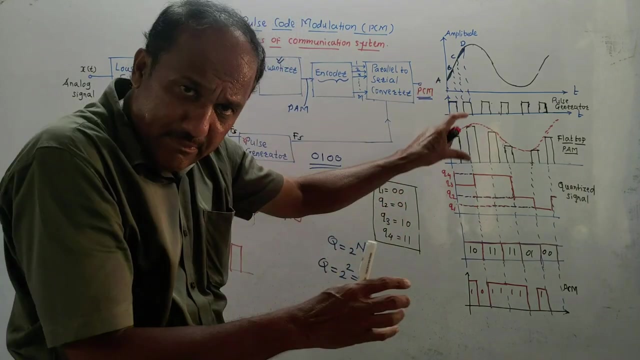 there's a deco you to pile up ocean. a first pulse. I'm talking about this pulse is kill, your suppose. does the ear pulse? a poor signal, co-homelow a little. a levels may divide carrying a. once again I will repeat your quantization of local detail. may learn carnival, a presently Jitna, recorded by 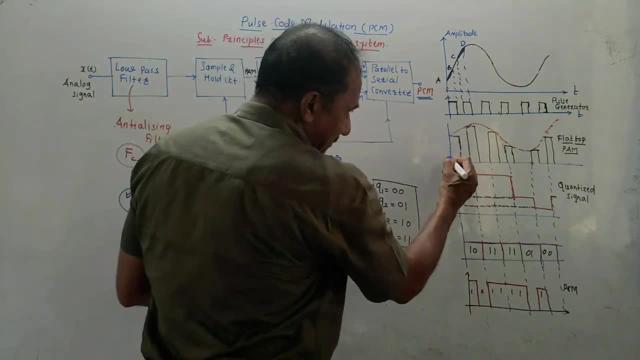 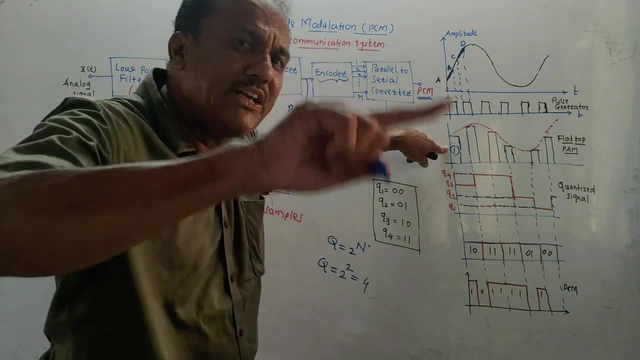 me. she topic takes print around, so there's a year per say. we will say this first pulse, I will say this first pulse. first pulse is, let us say it is around quantization level q3, so its value is assumed to be q3. to many a level is that? 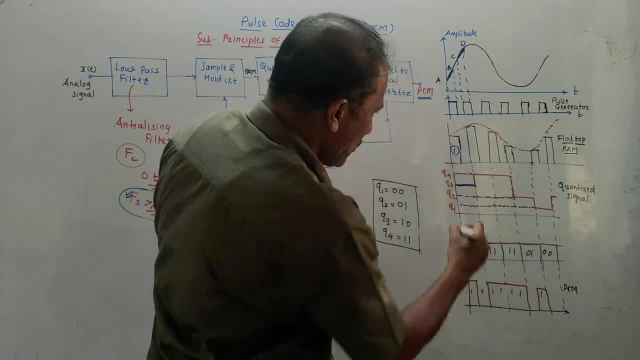 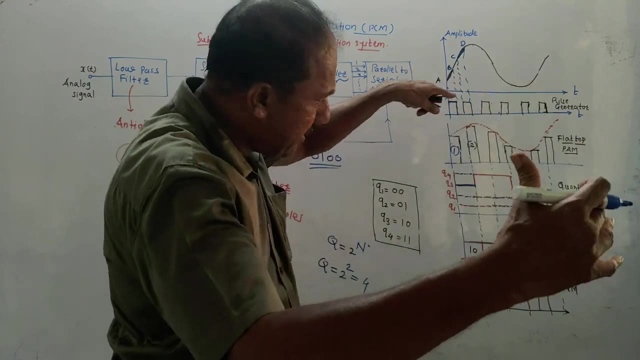 q3. drop here you Q 3 column second year you pulse a yes. second person say it is around. quantization level q4- yeah, around. or about approximate care of local detail will learn carnival is the height is at a isley is compensation level q3. 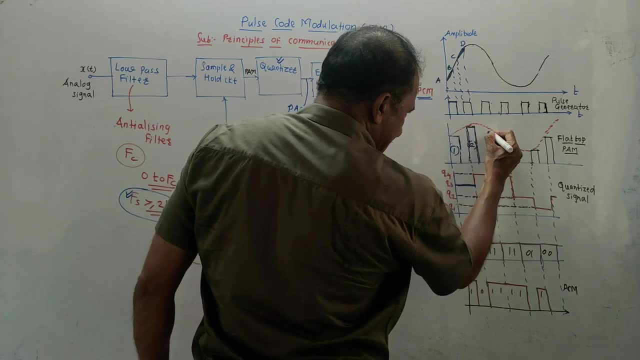 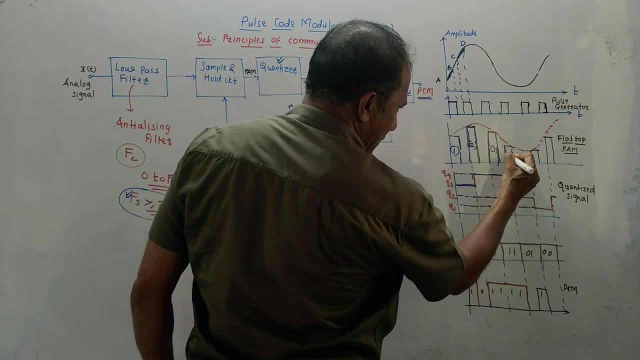 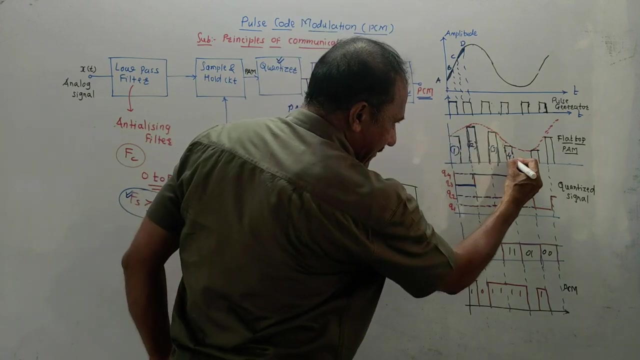 said: let us say it is q4, it's got a approximately q4. consider carrying a pulse number three: car to in the local quantification level: man, acid rock, yeah up your next next step. fourth pulse: yep, a little say, become high. so it is smaller pulse compared to all. it's the quantization level, my q2, I don't go. 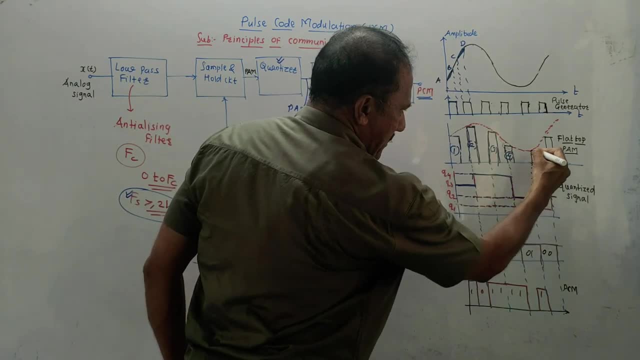 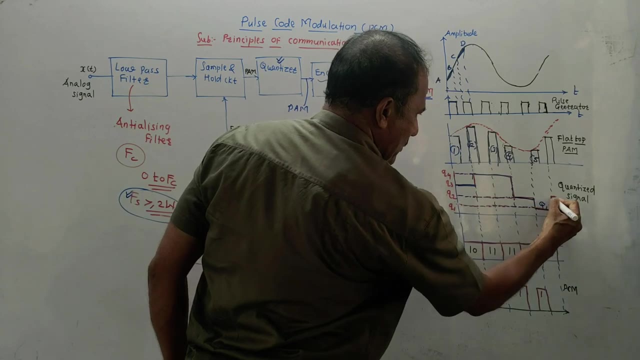 about the q2, but I'll be a level. likewise your job also is compensation level. I'm not q1, I don't get fifth pulse, so this is level q1. likewise we will be joining all the labels. ye jo, signal a, it is called quantage to signal. 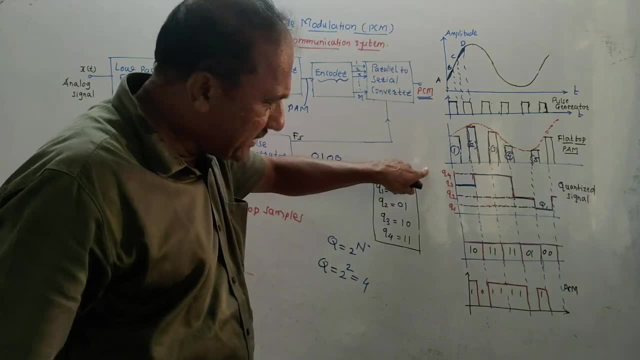 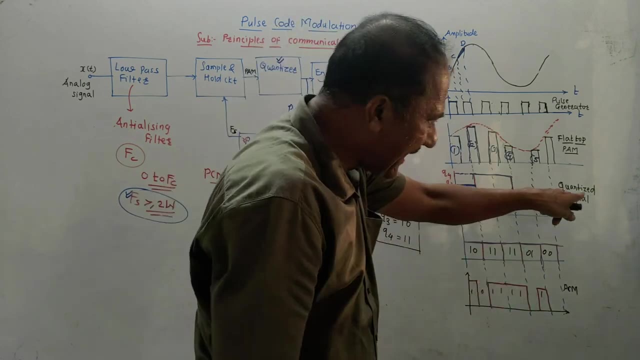 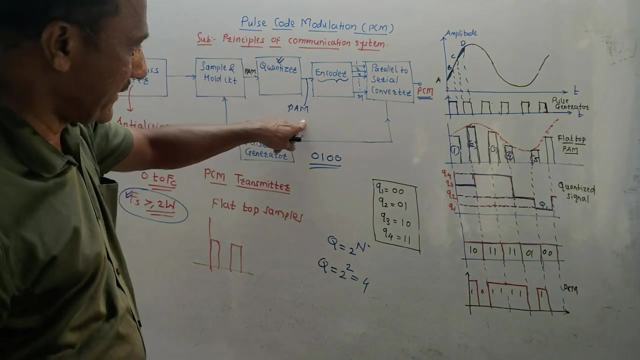 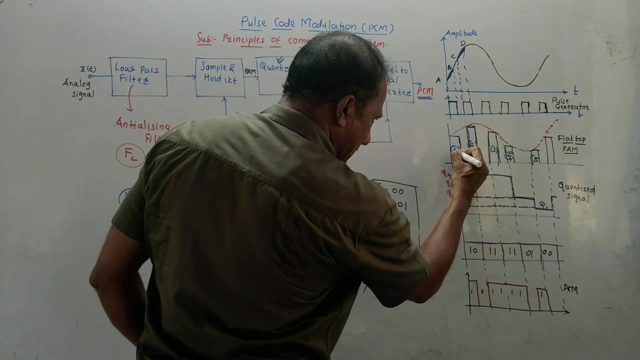 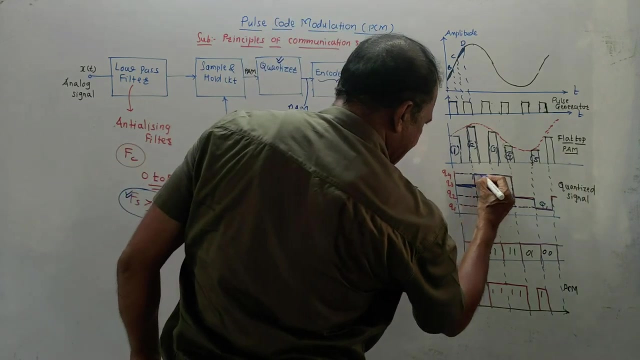 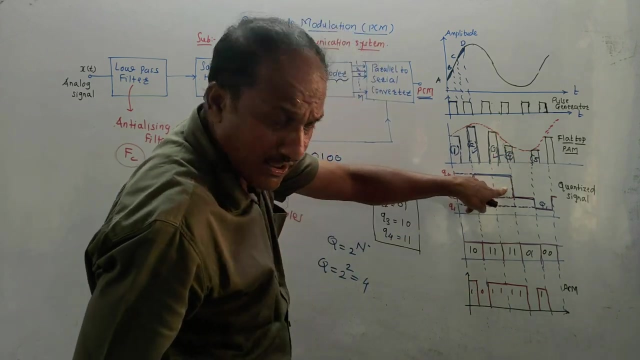 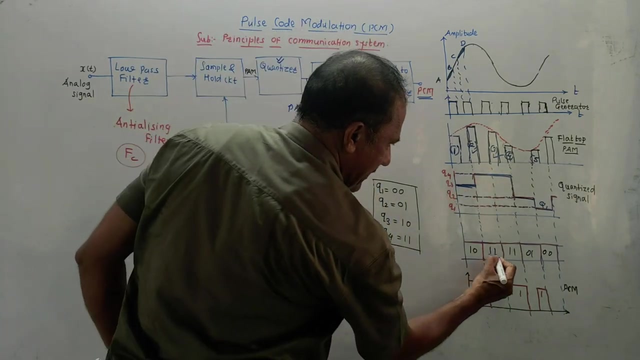 oh yeah, levels que se aggiunya calculation, cash in move will be going to discuss in our little ladder, ok, but so presently this is the output of contrast signal or output or quantizer block digital. today's core content of a B deliberative. The first level is Q3, the first level is related to pulse number 1, for Q3 the bits are 1, 0, so I have written 1, 0,. the second one is related to Q4, this is actually two slots: second pulse and third pulse. so this is second and this is third pulse. for this level, we have assumed Q4 for second and third, so Q4's value is 1, 1, so I have written 1, 1,, 1, 1,. this is Q2, this part. 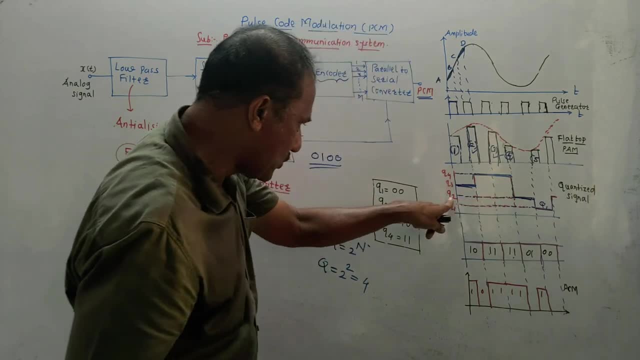 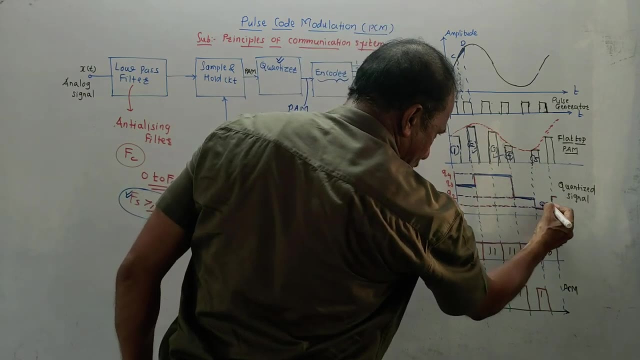 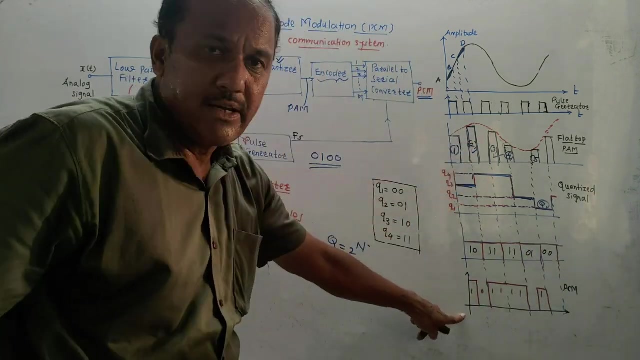 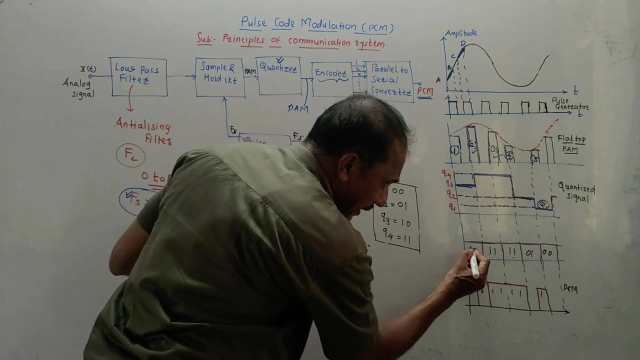 for fourth. for fourth it is level- is Q2,. look at Q2's level. look at Q2's value. look at Q2's bits 0, 1, here I have written 0, 1, last. for this we have assumed Q1 level of quantization. look at Q1's bits 0, 0, so I have written 0, 0,. last diagram: it is the actual diagram of code word that is output: PCM. this is very simple. look at the first combination: 1, 0, so the first bit is 1, the second is 0, 0 means 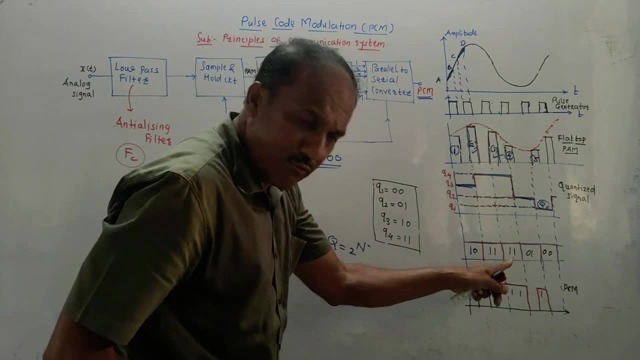 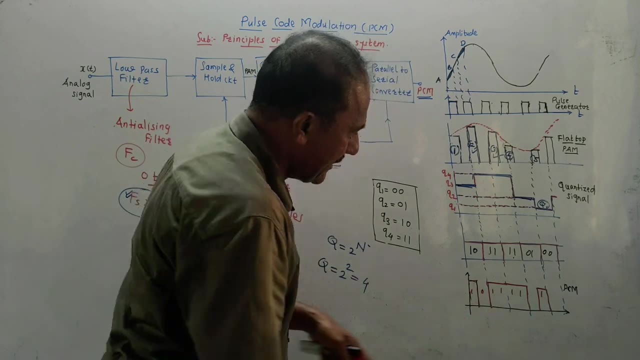 we will show the gap then four times. we are having 1, four times. so four times 1 is there. so we have shown the level high. it is very simple: 1 means high level, 0 means no signal. 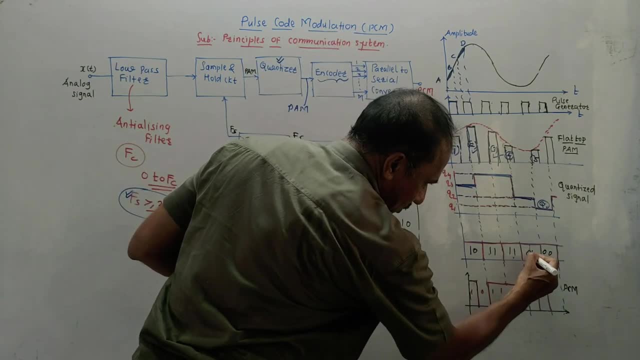 this first part is 0,. 2nd part is 1,. so this part has been divided into two parts. the first part is 0,. 2nd part is 1, here too, this is 0,. this is 1,. like this is divided into two. 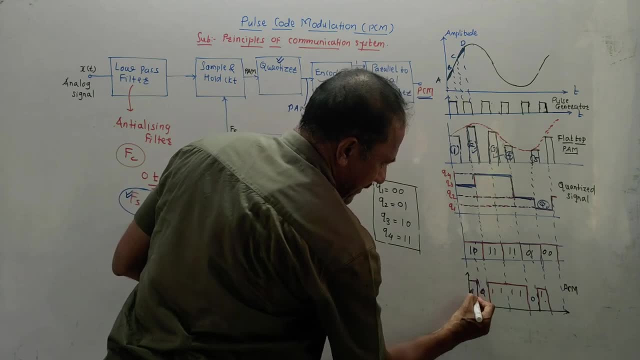 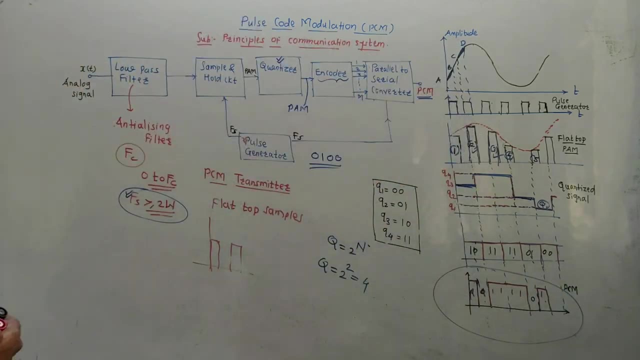 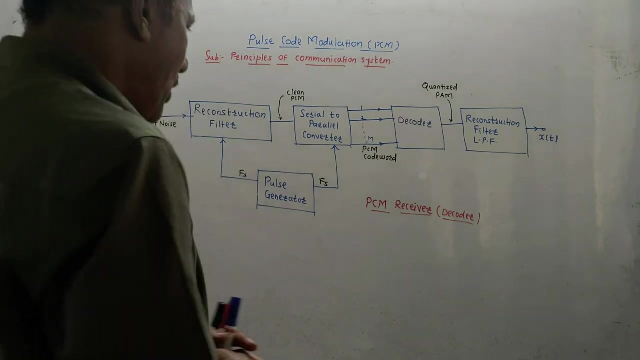 parts. so this is the first part. 1 is there, the second part is 0,. likewise 0, 0 is there. so we will not draw anything here. so this is the output, which is generally the output uh called the pcm, that is, pulse core modulated signal. next is the block diagram of pcm receiver. 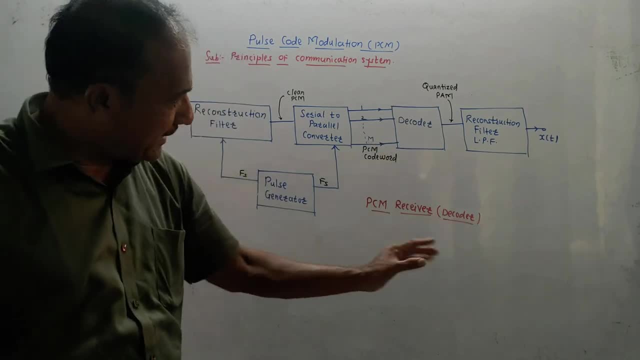 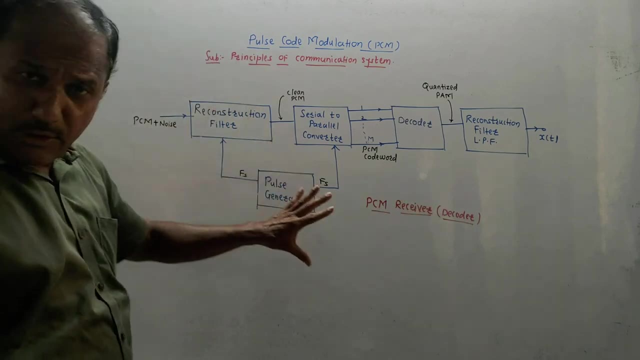 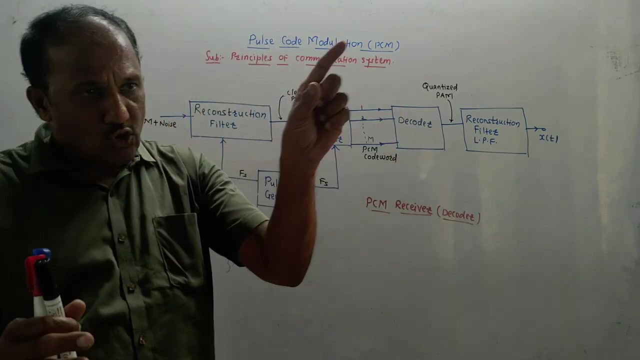 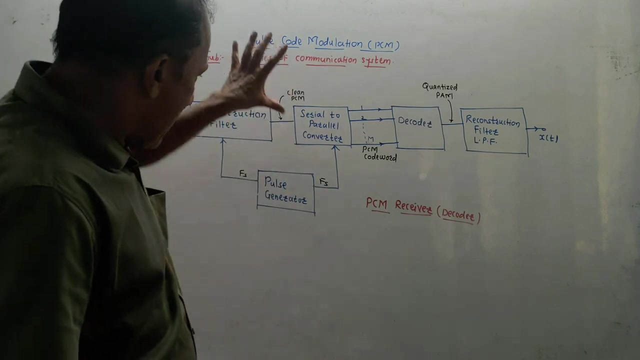 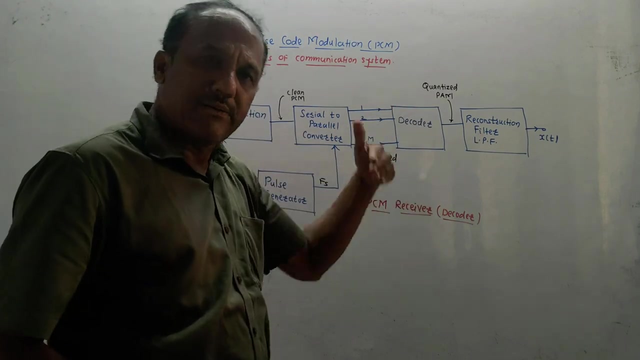 it is also called pcm decoder. it performs exactly reverse operation compared to the pcm transmitter. the final output we got in the transmitter was in terms of encoded signal. the function of decoder and receiver is to capture the encoded signal and convert back into the original form, convert back into the analog signal. 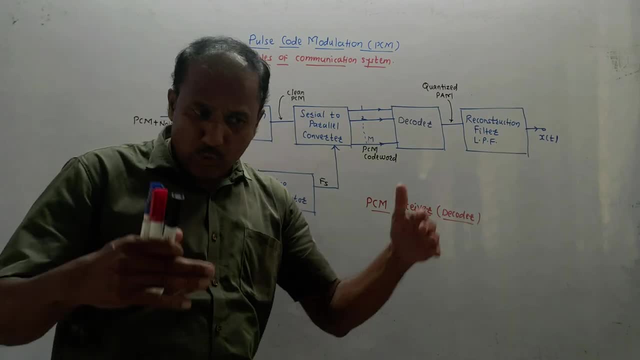 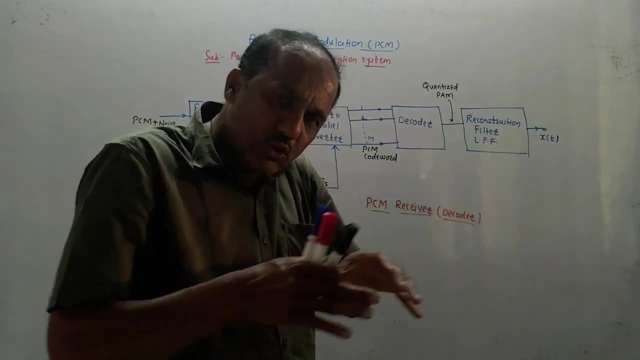 in case of transmitter, the output is codeword. these codewords are transmitted through some channel. what is channel? channel is a device through which channel is a medium through which the signals are passing. so codewords are transmitted through the medium, through the channel. 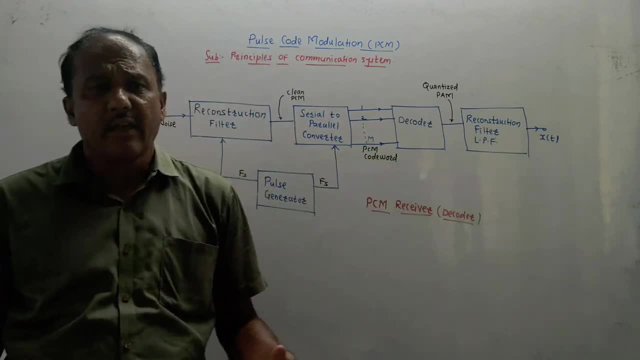 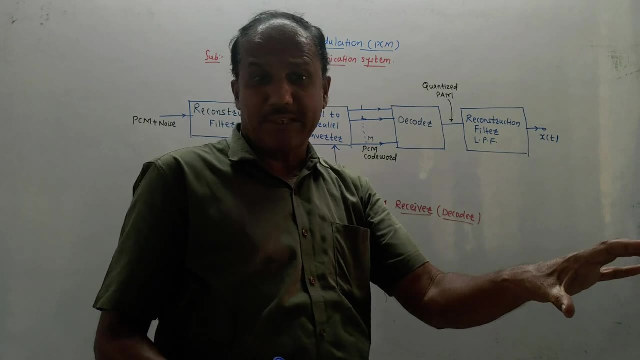 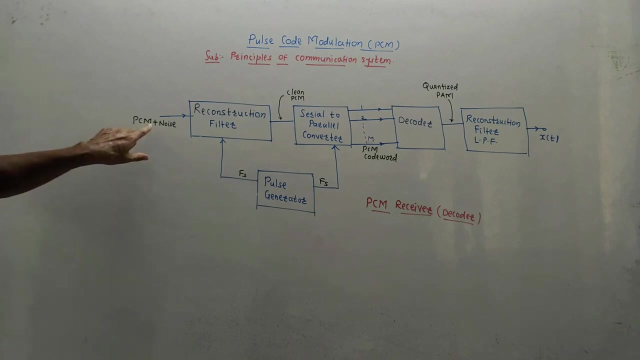 but the noise is getting added. now see, practically many generators are used in between in order to avoid the effect of noise. still, some noise is present. so at the receiver side this signal- i have written it as pcm plus noise- means pulse core modulation plus noise. actually, this is the output of transmitter side. 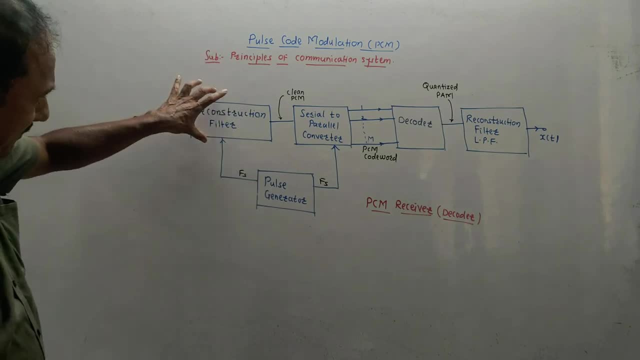 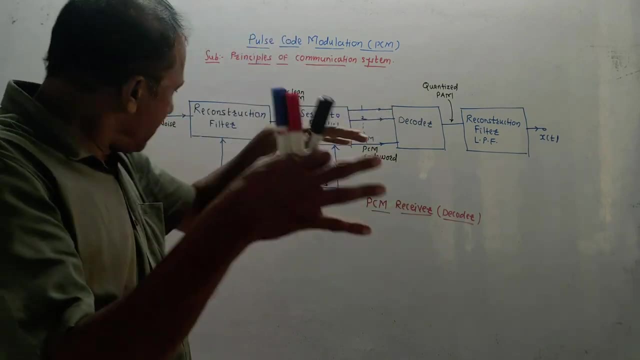 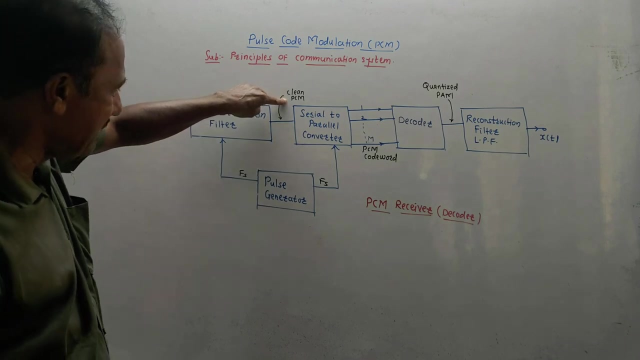 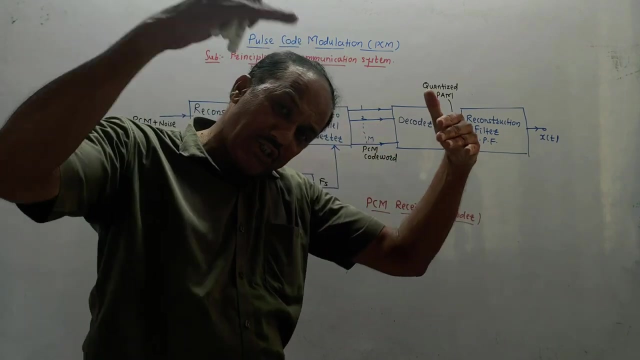 first block is reconstruction function. function of this filter is to reconstruct the signal means. in simple language, its function is to cancel the noise, which was included in this. so output of this reconstruction filter is clean or clear pcm signal. now next block is serial to parallel converter. it is exactly opposite to what we studied in transmitter. 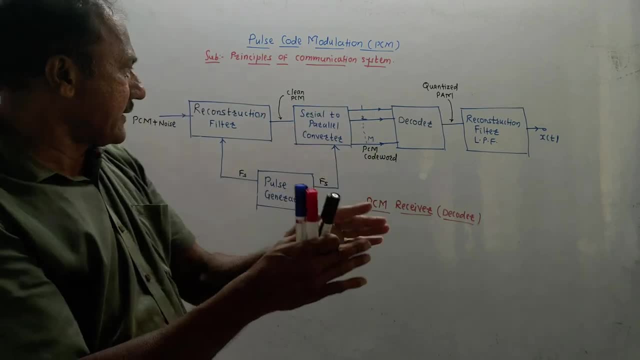 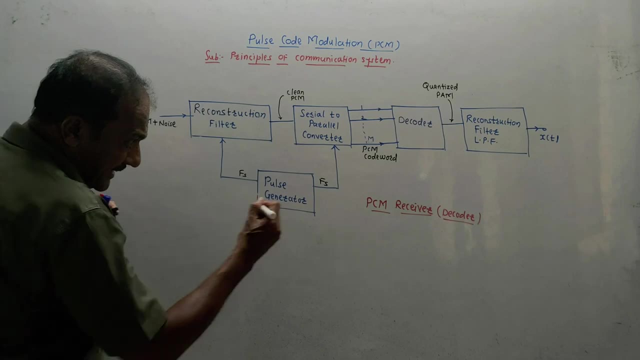 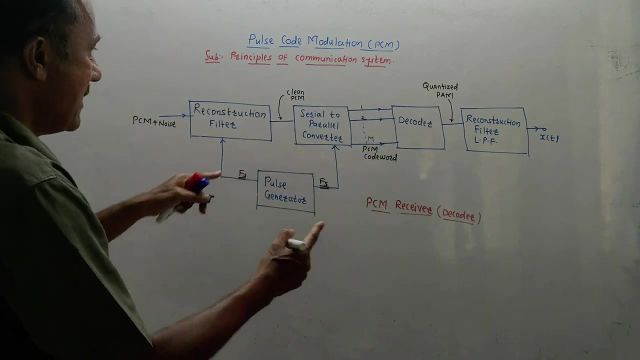 in transmitter we convert parallel to serial. here we are doing serial to parallel conversion because this is a receiver block. now see here this pulse generator is connected. its frequency is fs. this is the same frequency which we used in the transmitter. so serial to parallel converter, as the name indicates. 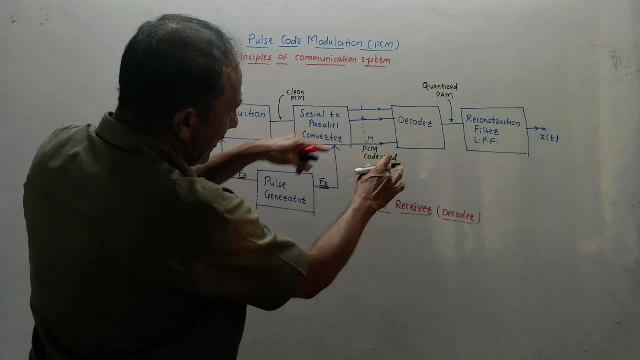 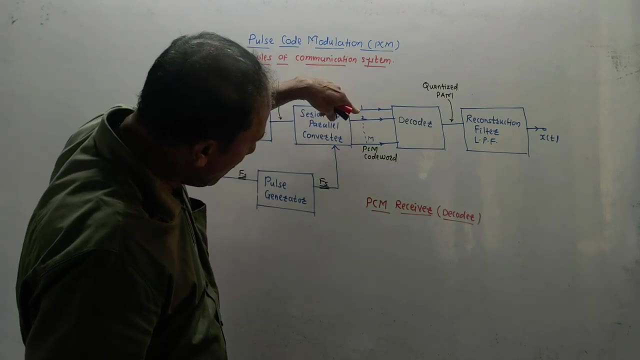 convert the signal into the parallel form. so in its output we will get parallel levels. it is pcm codeword which will be in the parallel form, having codewords from 1,2,3 upto m, so it is m pcm codeword. next block is the decoder. as the name indicates, it decodes the signal. decoding means exactly opposite operation, like we discussed in transmitter. all the quantization levels. quantization means approximation, all the approximation levels. we have assigned codeword to all the levels. function of decoder is this: convert this pcm codeword into quantized level. 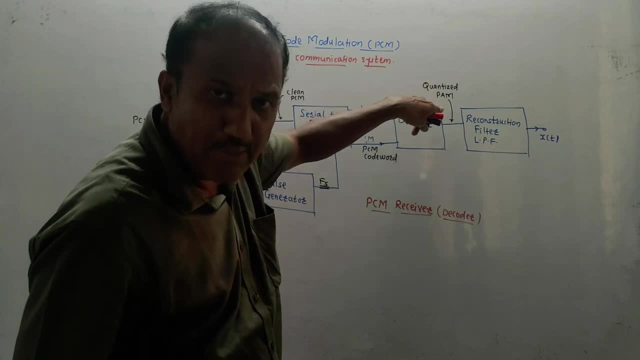 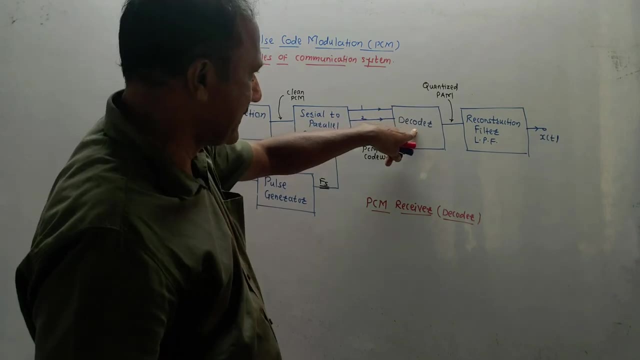 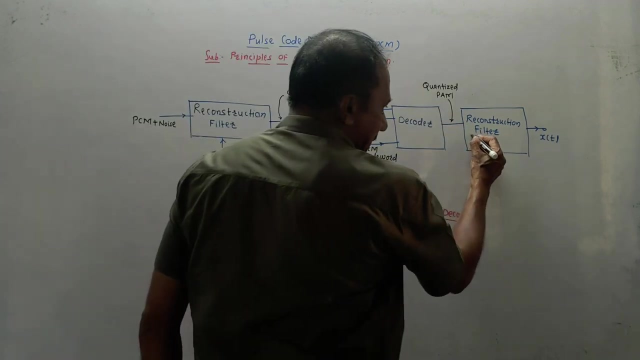 this is so output of decoder. this decoder is quantized PAM to keep in mind. it is very simple. the operation is exactly opposite to that we performed in transmitter session. then this quantized pulse amplitude modulation signal, PAM signal, is given to the reconstruction filter. it is basically low pass filter. 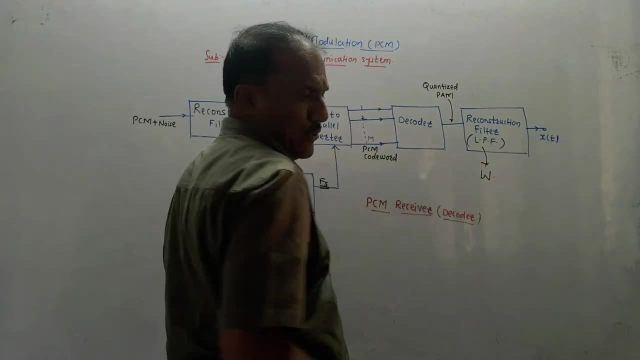 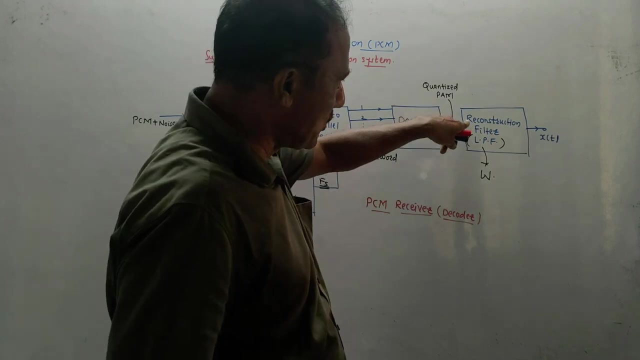 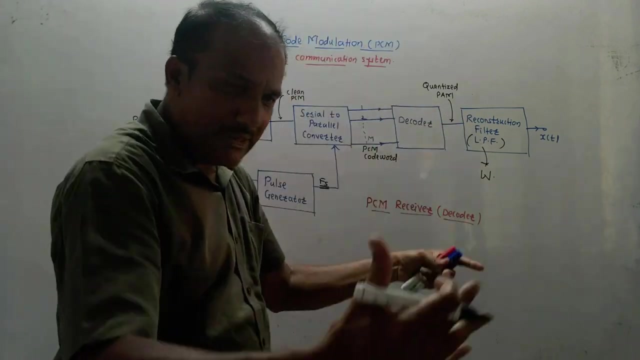 it has cut off. frequency that is kept. equals to W means W 0 to W signals will be passed. the signals which are above W will be blocked. so this is the function of reconstruction filter. make it simple. reconstruction filter means the final output that should be same as or exactly replica. 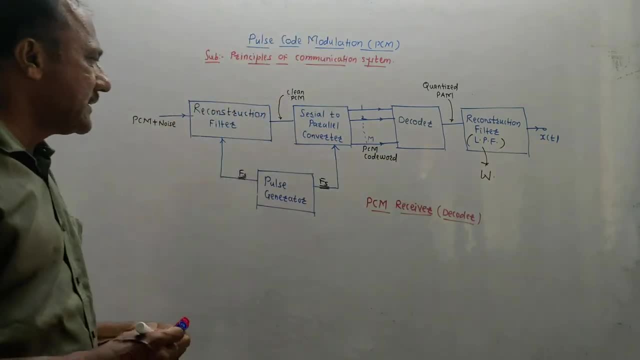 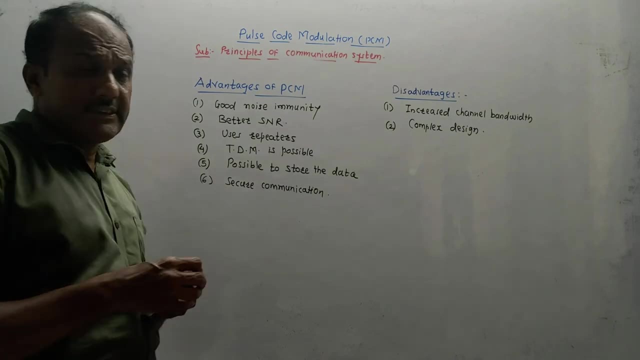 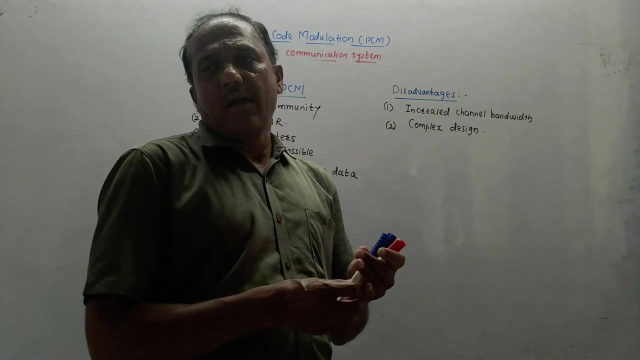 of the original signal. so at the output you are getting signal X of t. so this is the block diagram of PCM receiver. now we will discuss advantages and disadvantages of PCM system. basically PCM system is used in digital telephony system, then in space communication and so on. 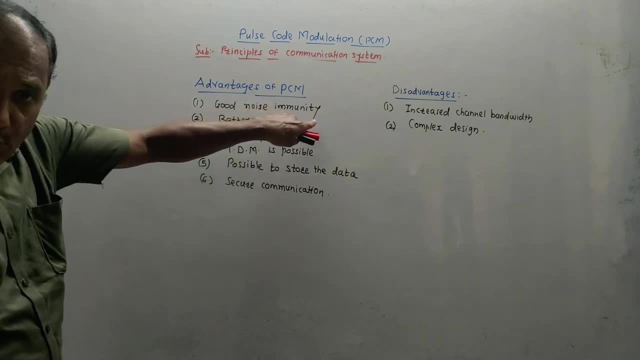 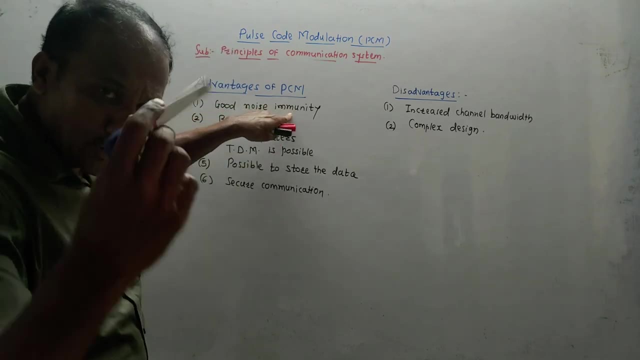 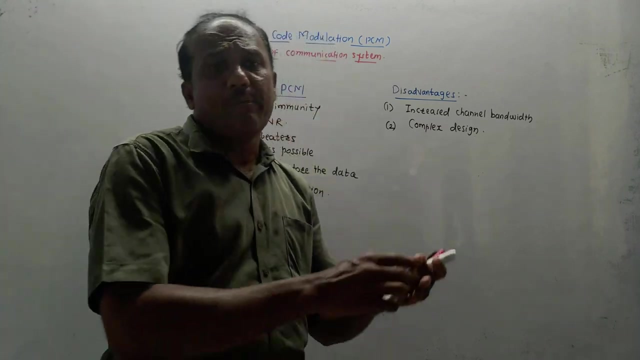 advantages are: it has good noise immunity. second, better SNR. SNR means signal to noise ratio, so noise immunity means opposition to the noise. this is better, so better signal to noise ratio is obtained. it makes use of repeaters, as I explained. many repeaters are used. 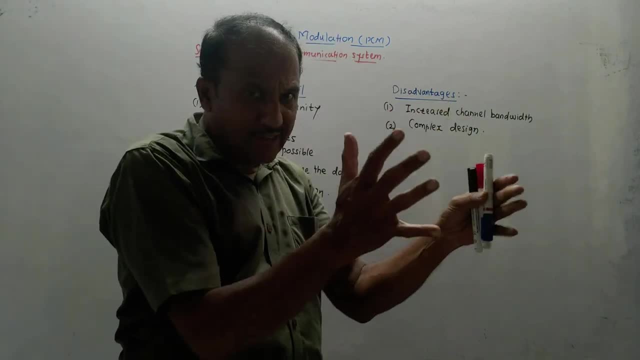 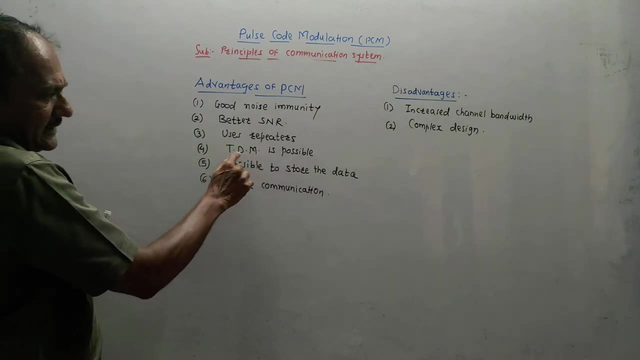 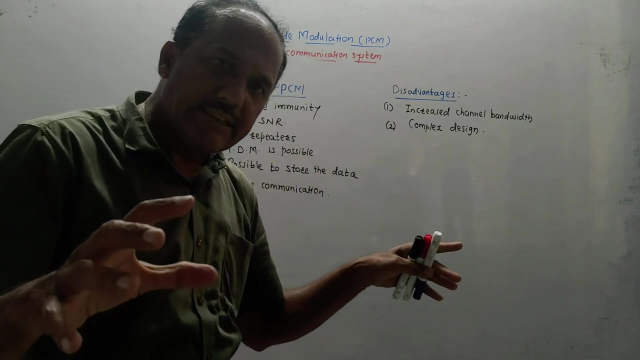 repeater is regeneration of circuit, so noise is eliminated at various stages. in case of PCM system, then time division multiplexing, that is, TDM time division multiplexing, is possible. next, possible to store the data. very simple, because the data is in the form of digital. 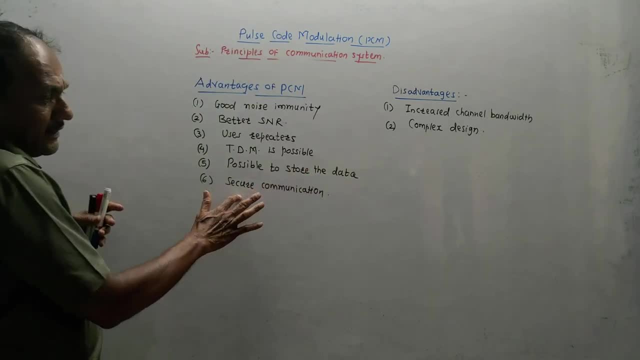 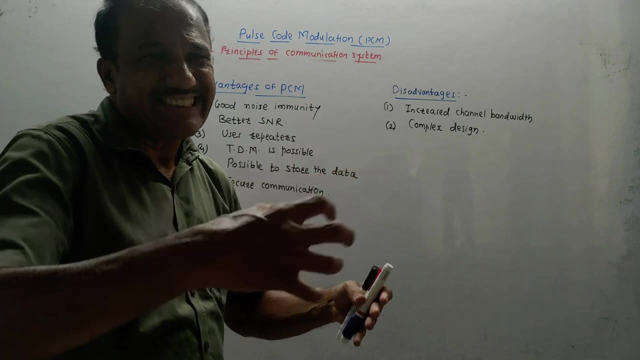 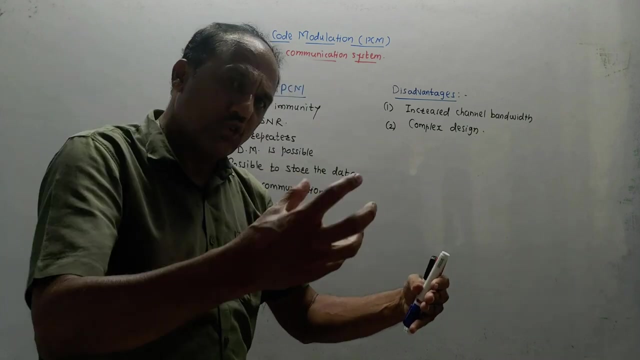 so you can easily store the data. and last, very important advantage is it gives secure communication. as we discussed, that output is in encoder form, so different coding techniques can be used. so while decoding, the person who will decode whose coding technique is known prior. so it provides secure communication. 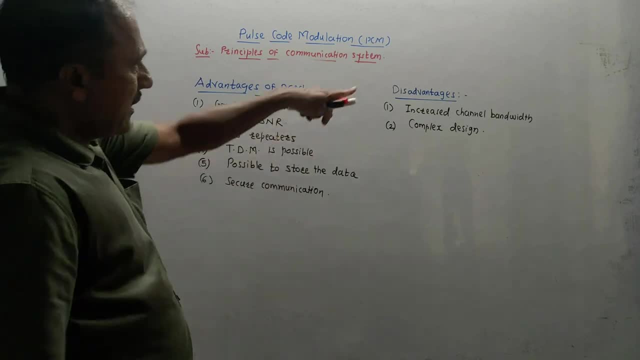 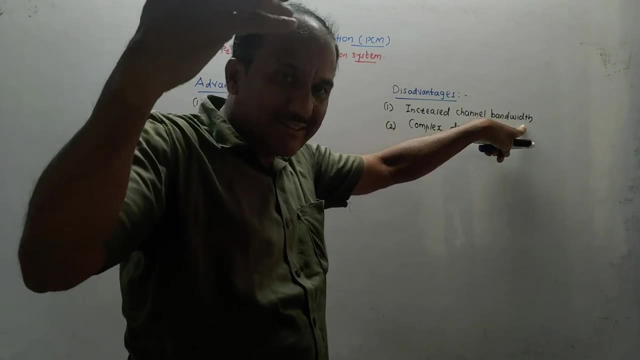 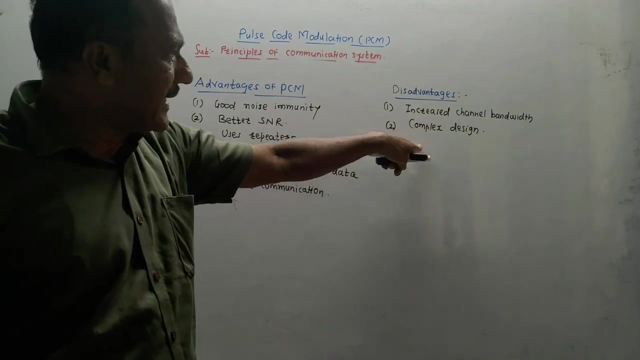 because any kind of coding technique can be used. disadvantages: increase channel bandwidth, like we will increase the quantization levels, like the bits which are used to represent every word. those bits will increase which will demand for more channel bandwidth. and second is the complex design. so these are few advantages and disadvantages.